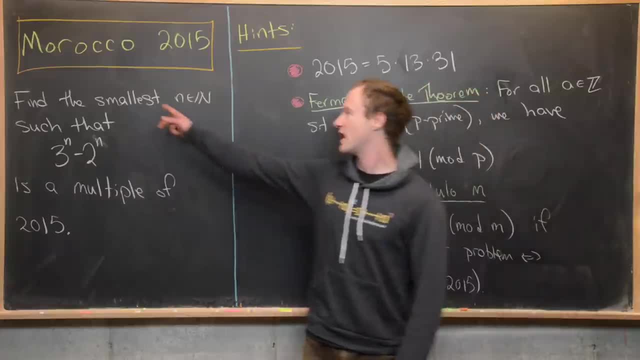 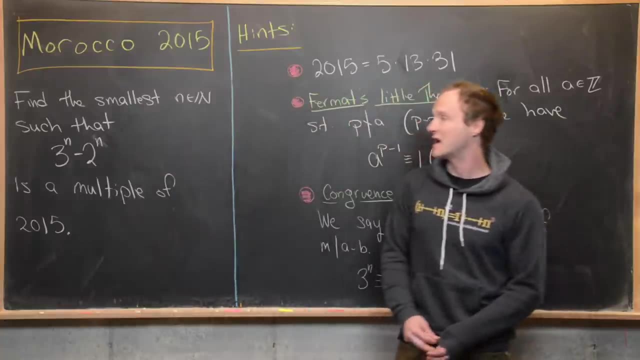 Okay, so let's look at the statement of this problem. We want to find the smallest natural number, and by natural number I mean positive integer, such that three to the n minus two to the n is a multiple of 2015.. So, in other words, it's divisible by 2015.. Okay, so I've got some hints. 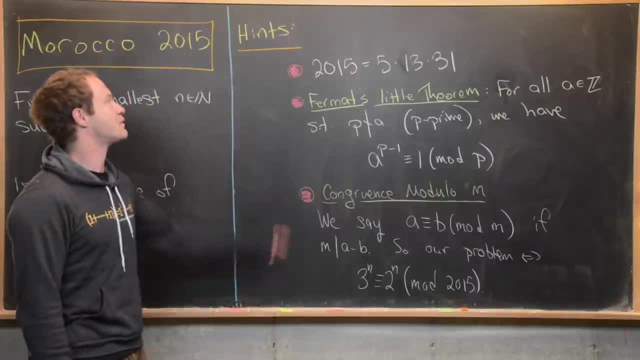 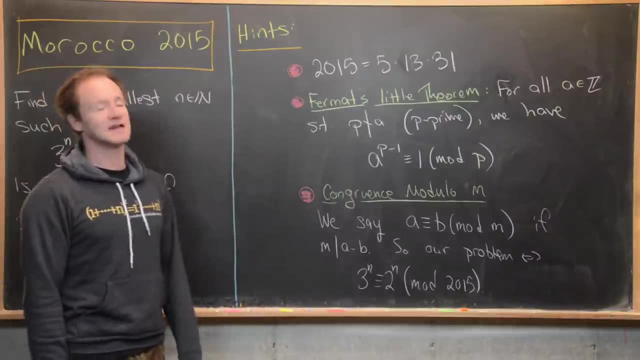 worked out, So you guys can maybe try this problem before we look at a solution. The first hint is that 2015 has the following prime factorization: So it's five times 13 times 31.. So whenever you're talking about divisibility, 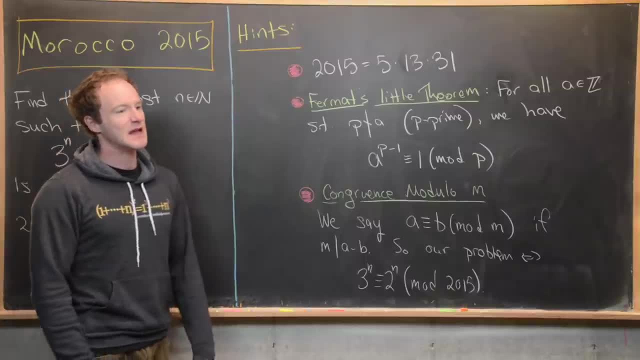 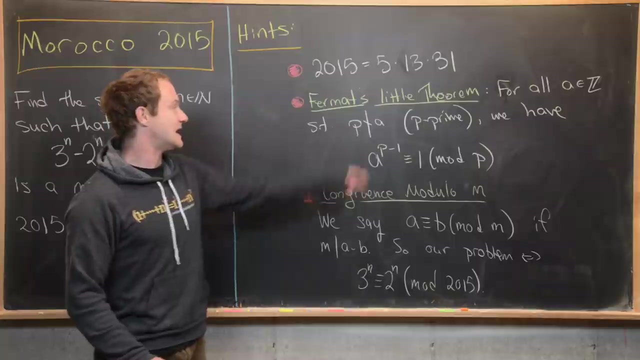 especially divisibility by a composite number. it is often helpful to look at divisibility by the component prime numbers. Then next there's this thing called Fermat's Little Theorem. that might help And that says that for all integers, a such that p does not divide a where p is a prime. 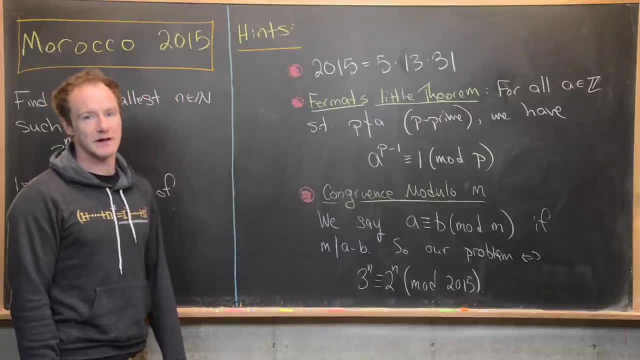 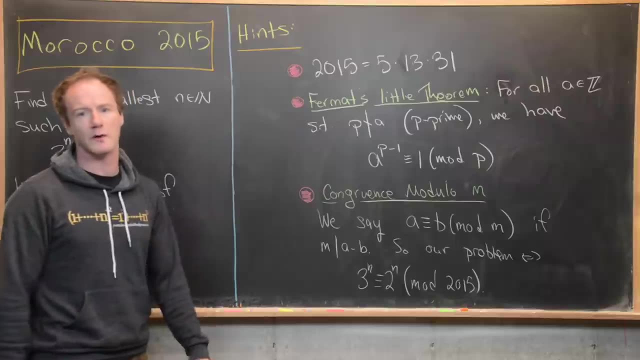 we have a to the p minus one is congruent to one mod p, And the fact that I've used the notion of congruence mod p Down here means that maybe we should recall what that means. So congruence modulo M, where m is: 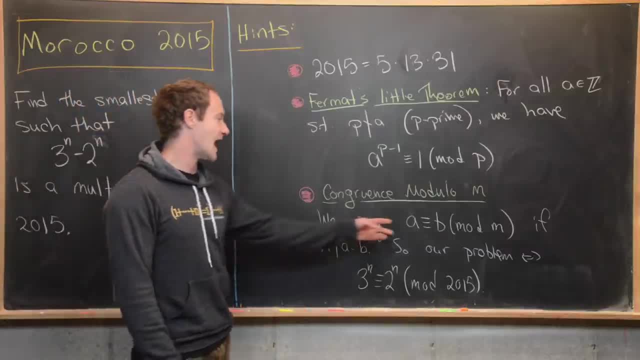 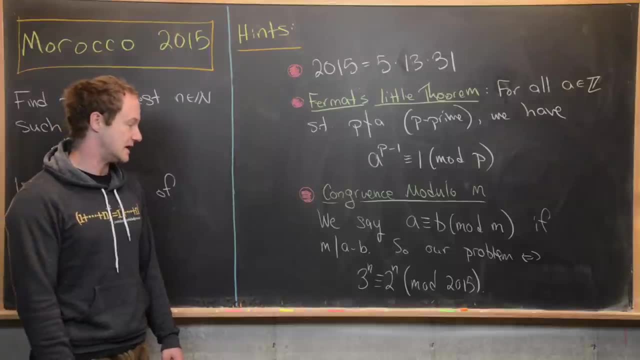 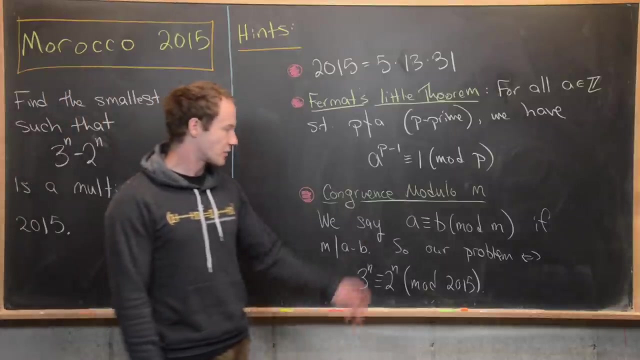 any natural number is defined as follows. So we say a is congruent to B mod M if m divides A minus b. So in other words, A minus B is a multiple of m, or a minus B is divisible by m. So our problem is: 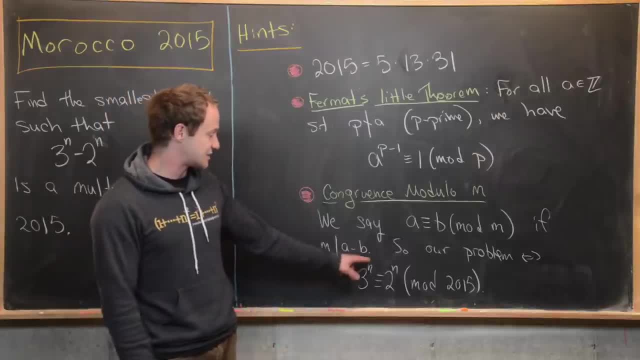 equivalent to finding an n such that p is a prime, And we've got to find a value in that value in the matrix. So that's why it's called the Fermat's Little Theorem. So we're going to go over to the 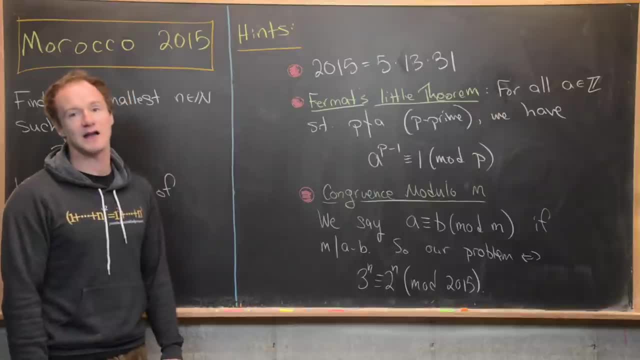 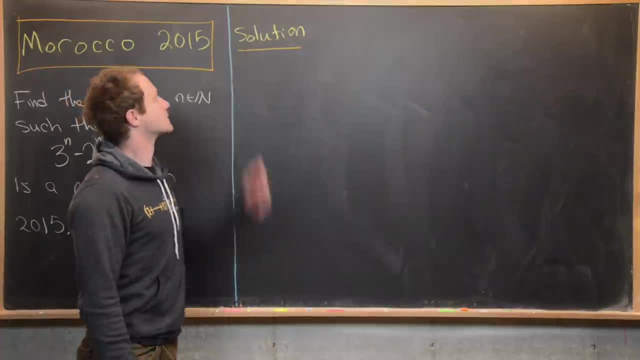 that three to the n is congruent to two to the n, mod 2015.. Okay so, maybe give this problem a go with these hints and we'll come back with a solution. Okay so, hopefully those hints were helpful. Now we're ready to look at a solution. 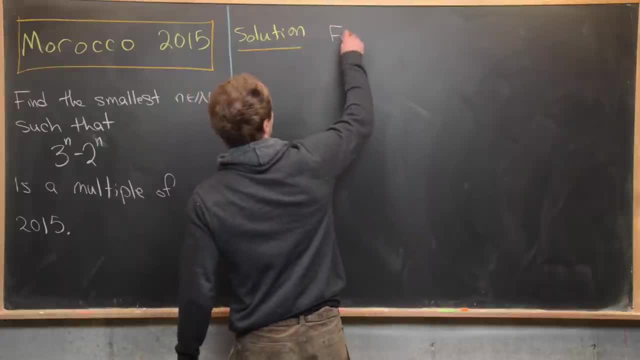 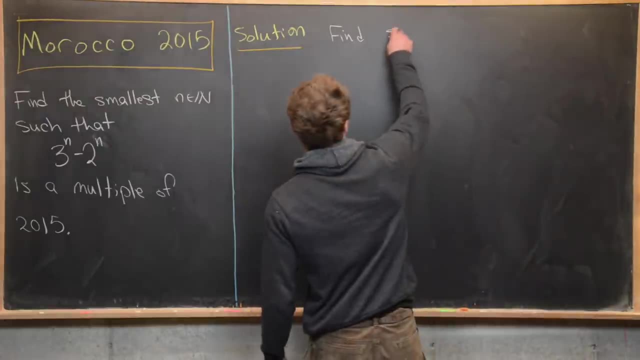 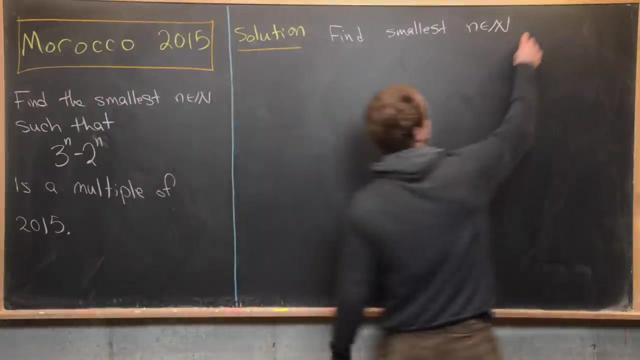 So I wanna translate this problem to the following problem, which is equivalent, via this notion of congruence, modulo m, which was described on the last board. So we wanna find the smallest natural number, ie positive integer n, such that we have three to the n. 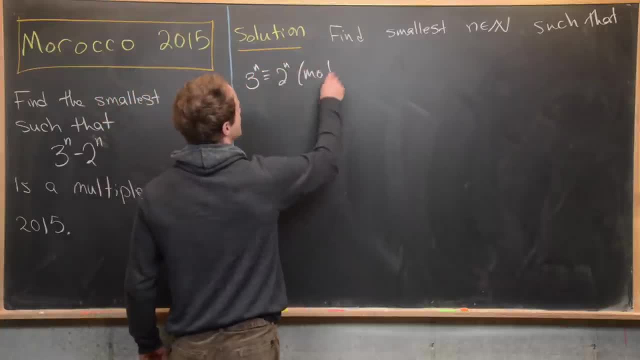 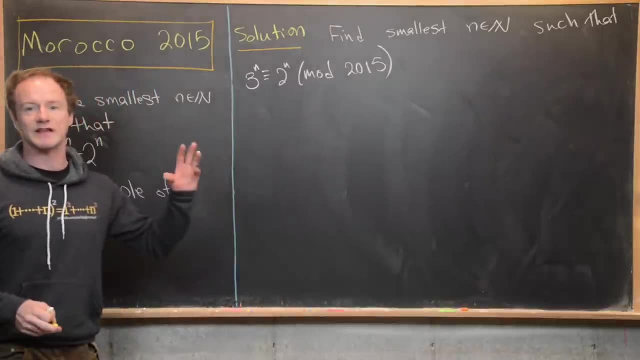 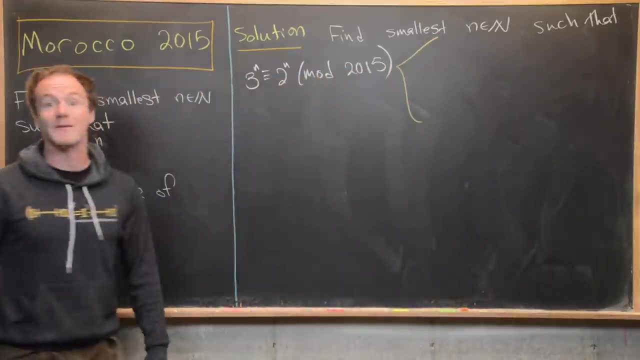 is congruent to two, to the n modulo 2015,. great, But now we can actually spread that out into a system of congruences, and that system of congruences will have to do with the prime factors of 2015.. So, like I just hinted at, 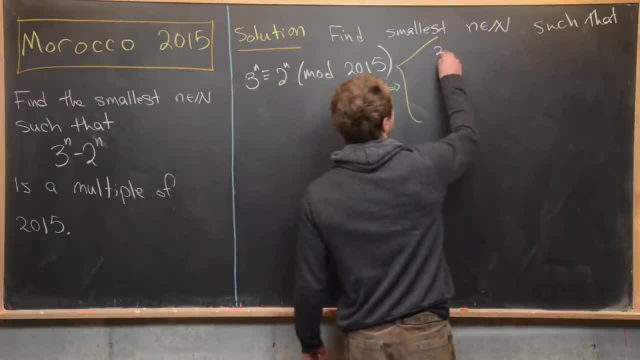 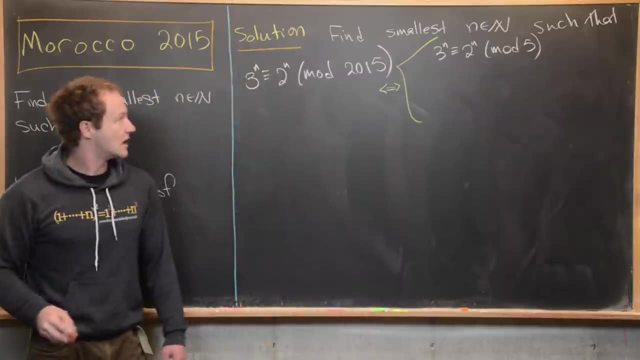 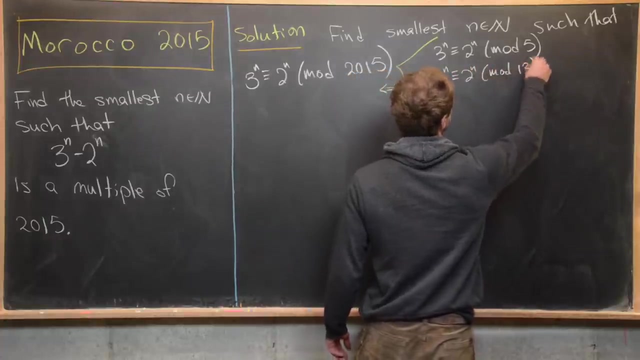 this is if, and only if, we have three to the n is congruent to two to the n modulo five. That would be the first prime factor of 2015.. And then we have three to the n is congruent to two to the n modulo 13.. 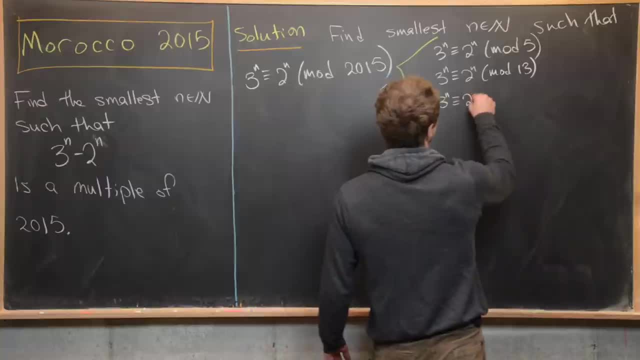 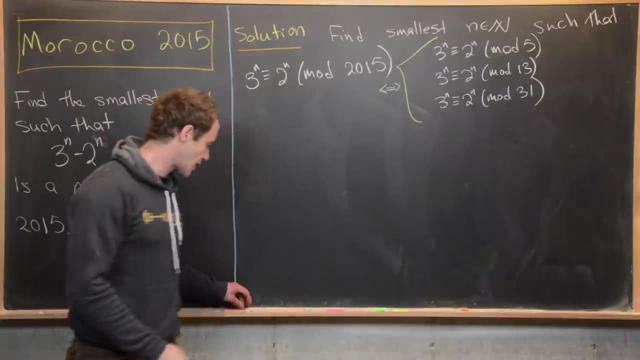 And then finally, three to the n is congruent to two to the n, modulo 31,. great, So now let's maybe work, let's see, let's see, let's see, Let's maybe work on each of these separately. 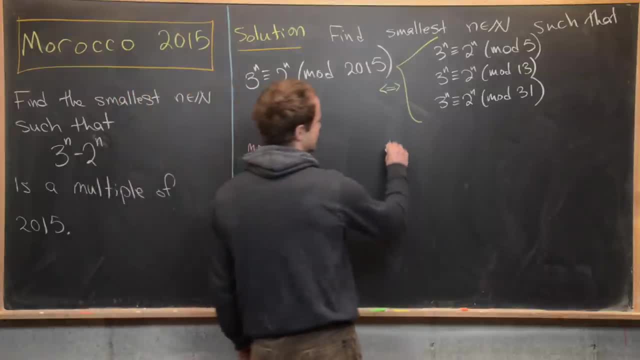 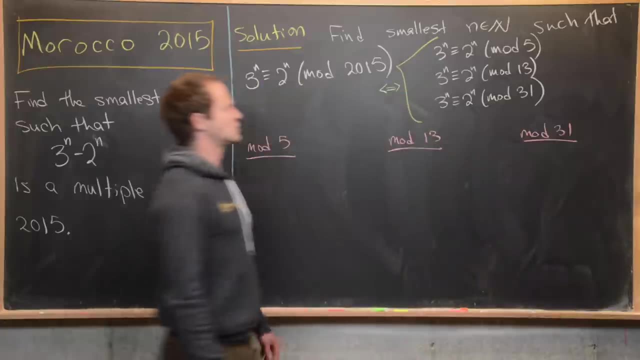 So let's maybe work mod five first, then we'll work mod 13,, and then, finally, we'll work mod 31. And then we'll try to mash all of these things together. So if we work mod five, notice that Fermat's Little Theorem. 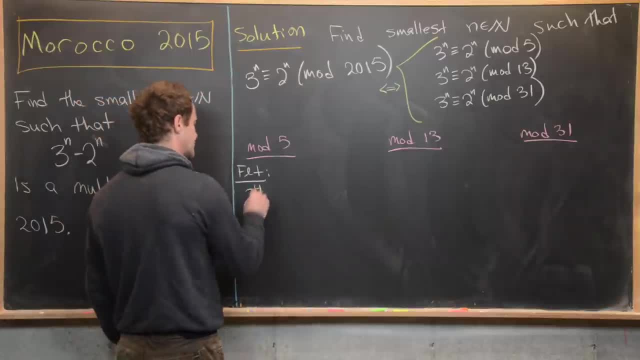 says that three to the five minus one, which is three to the four, is gonna be congruent to one mod five. But then two to the four is also congruent to one mod five Again, because two and three are not multiples of five. 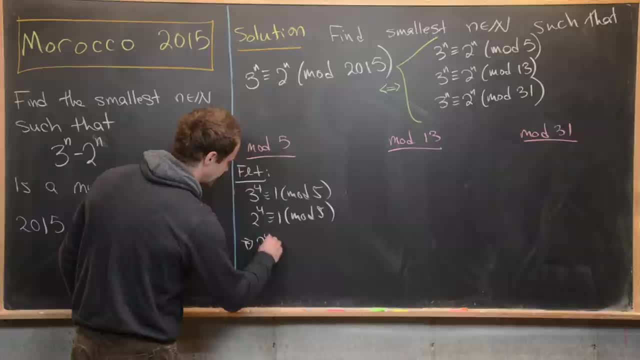 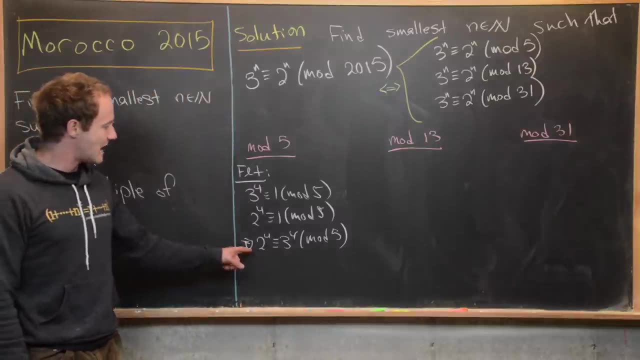 But what that tells us is that two to the four is congruent to three to the four mod five. And you might say, well, maybe they could also be equal without both being congruent to one mod five. And that actually happens in this case. 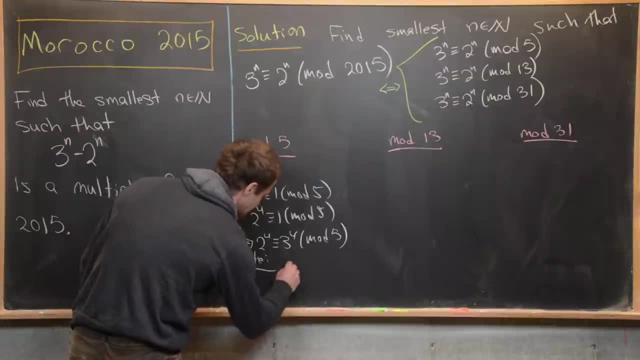 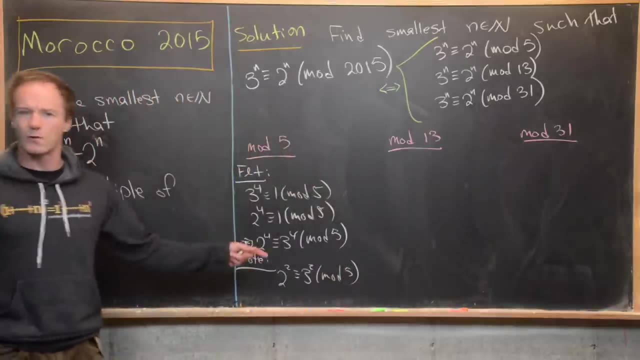 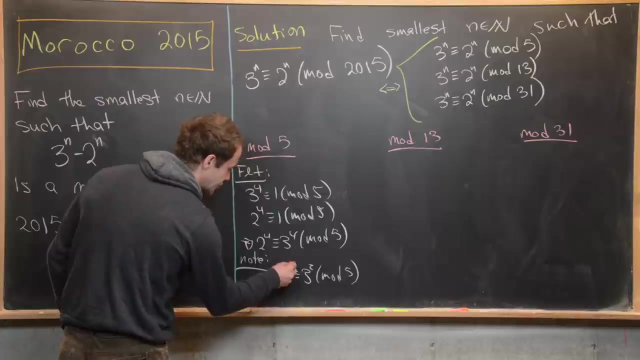 So let's notice that we also have two squared is congruent to three squared mod five. And so two squared is four, three squared is nine, but nine is congruent to four mod five. But the important thing here is that two is one of the divisors of four. 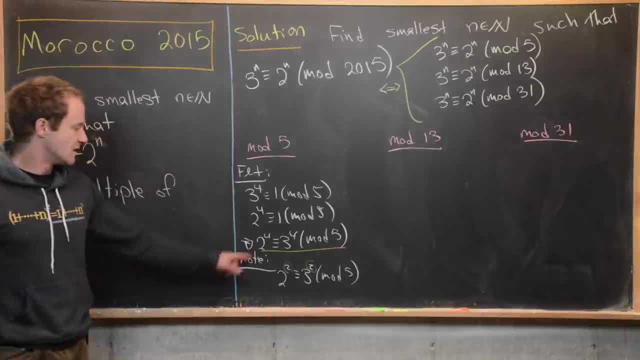 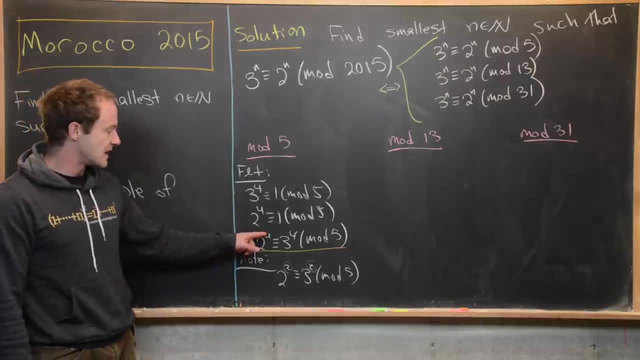 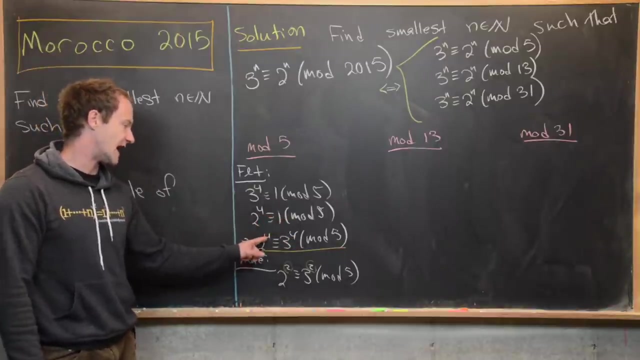 So if we get this kind of fact happening for some number right here, then we can prove- and this is actually how we'll finish the solution off- we can prove that the only types of numbers that are smaller that could also provide this result are the divisors of this exponent. 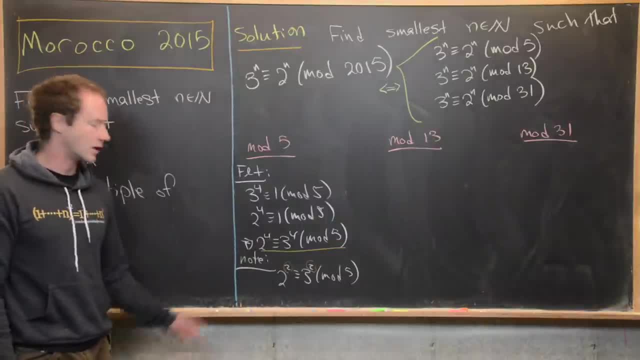 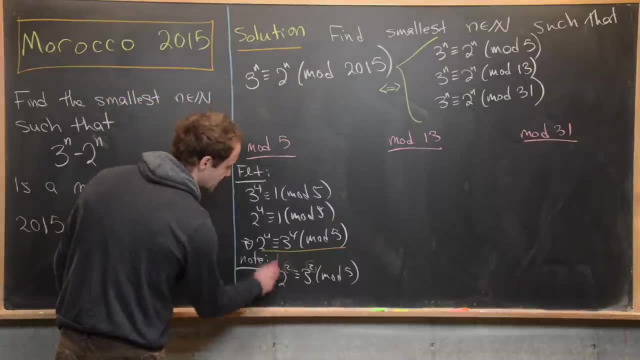 So in this case, the only number smaller than four that could provide this result would be one and two, because those are the divisors of four, And we see that, yeah, in this case two works. So here we have two to the two is congruent. 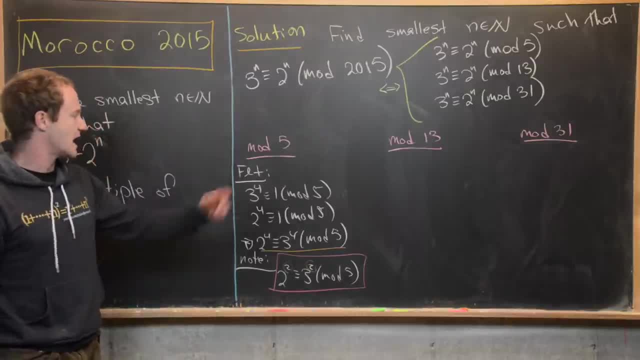 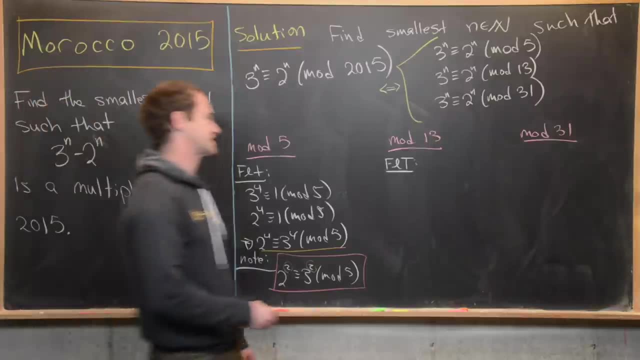 to three to the two, mod five. Now let's go ahead and work mod 13.. So again, we're gonna start with Fermat's Little Theorem, which will say that three to the 12 is congruent to one mod 13,. 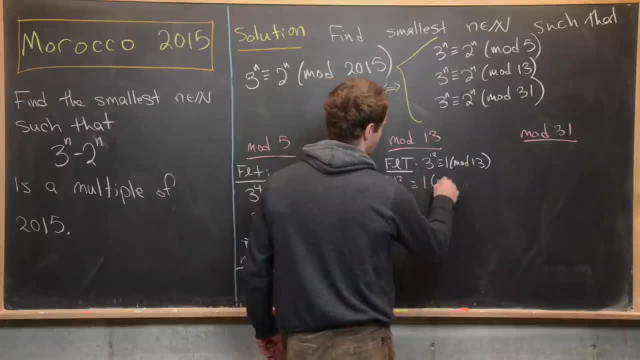 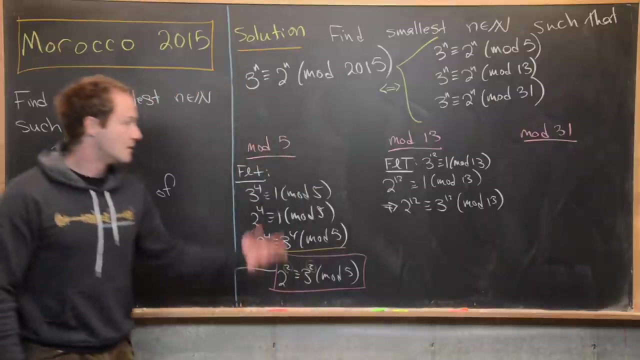 and two to the 12 is congruent to one mod 13.. Great So, but that tells us that two to the 12 is congruent to three to the 12 mod 13. But that's not necessarily the smallest number that allows for this congruence. 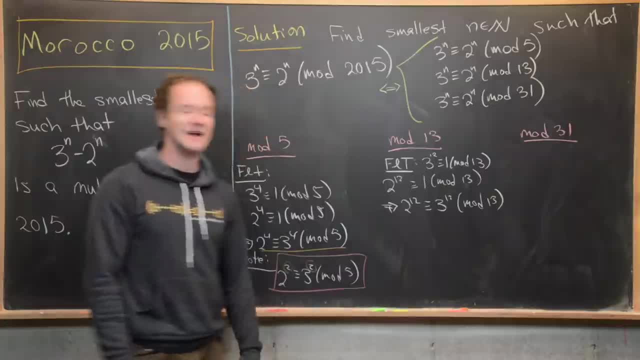 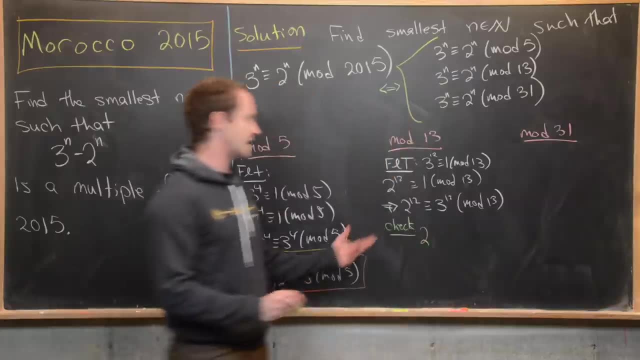 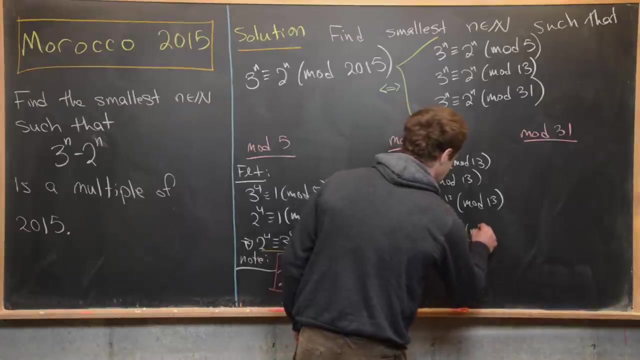 We could also have solutions that are divisors of 12.. So we would also need to check the following: So two to the well, what are the divisors of 12?? We could check. two to the six. is that congruent to three to the six, mod 13,? and we could check two. 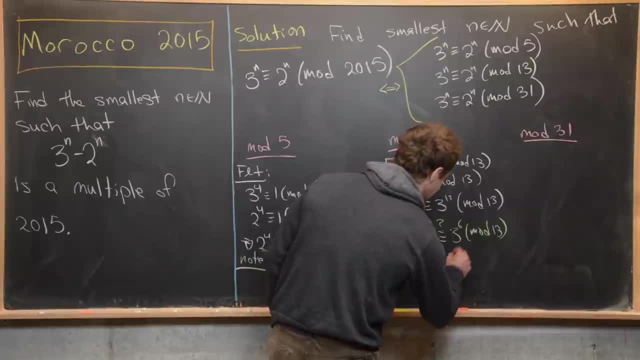 to the four. is that congruent to three to the four, mod 13.. So that's another divisor of 12. We could check: two to the three. is that congruent to three to the three, mod 13,? and so on and so forth. 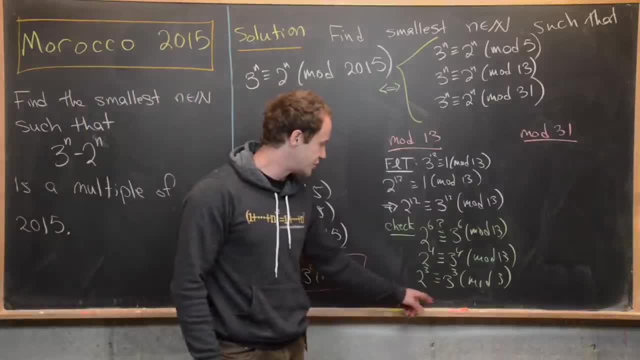 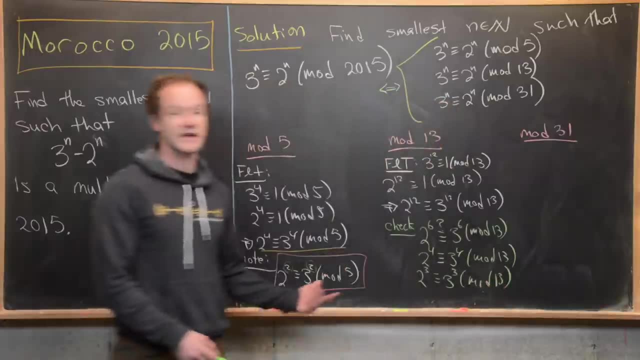 Well, let's maybe check some of these really quickly. So notice that two to the three is eight mod 13.. So two to the three is eight mod 13.. But three to the three is 27,, which is one mod 13.. 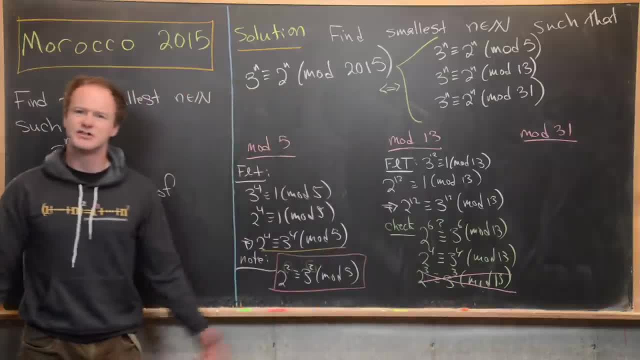 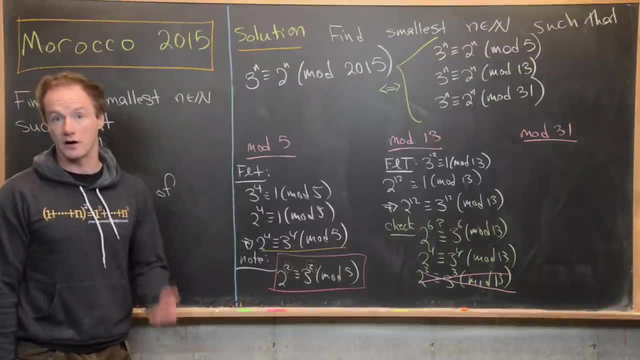 So this congruence does not hold. And then two squared and three squared. well, you can check that that congruence does not hold either. Notice: four and nine are not congruent, mod 13,. but I don't really have room to fit that in here. 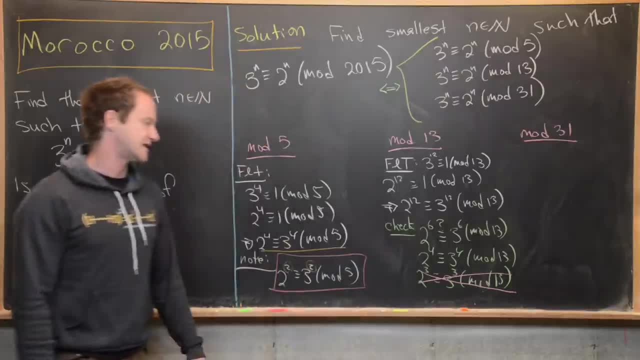 Then the next thing that we can do is maybe check this two to the six and this three to the six, But notice two to the six and three to the six. they are both, but notice two to the six and three to the six. they are both. 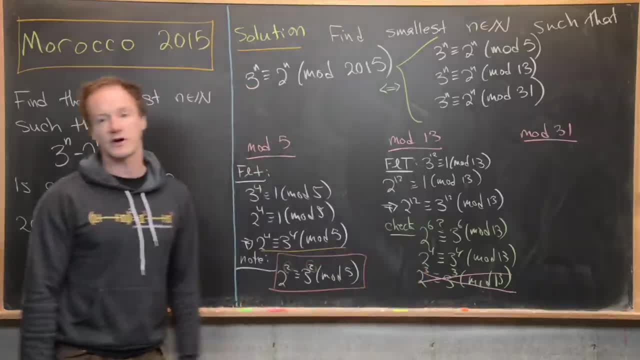 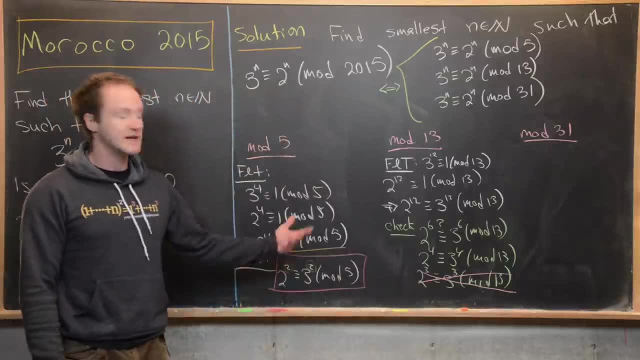 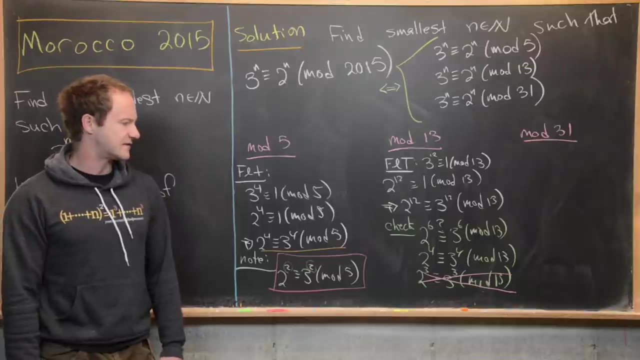 both equal to two cubed squared and three cubed squared. So recall that this was eight and this was one. but if we square eight mod 13, we will get 64.. But notice that 64 is in fact negative, one mod 13.. 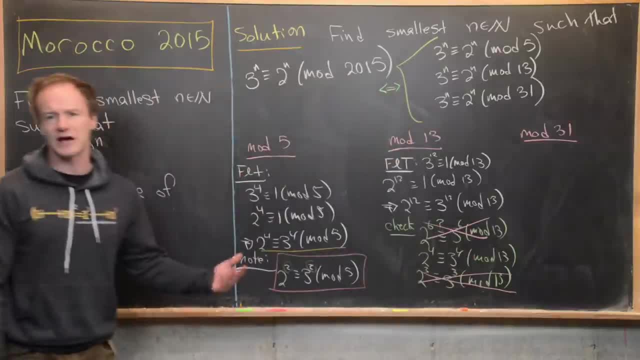 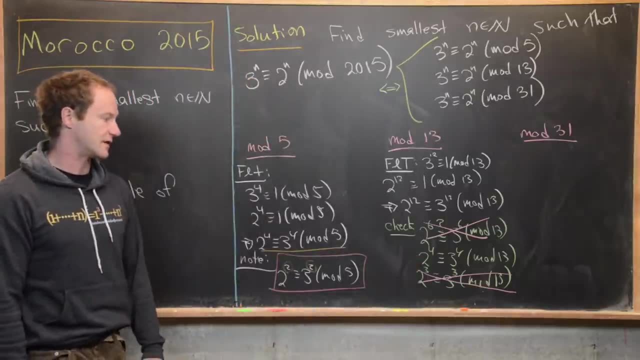 So this does not hold either. So I'll let you guys check that as well if you wanna work out all of the details. But you can check this thing in these. these are congruent mod 13.. So two to the four is equal to 16,. 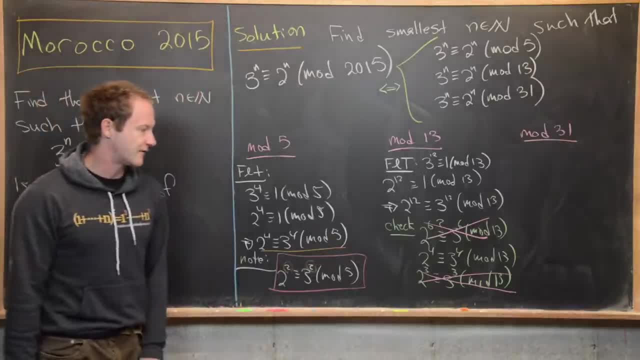 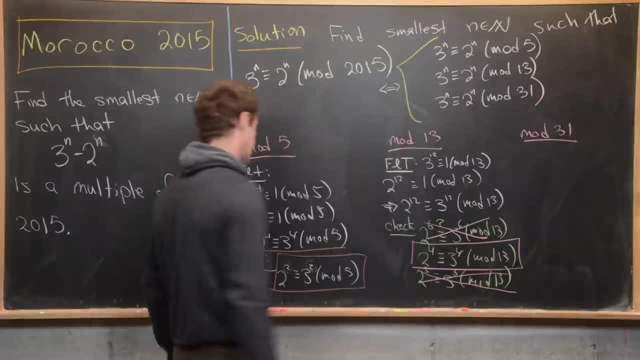 but 16 is three mod 13, and then three to the four. well, that's 81, and that is also three mod 13.. So this one is okay. So we've got a congruent solution there. So notice, if we put these two facts together at this moment. 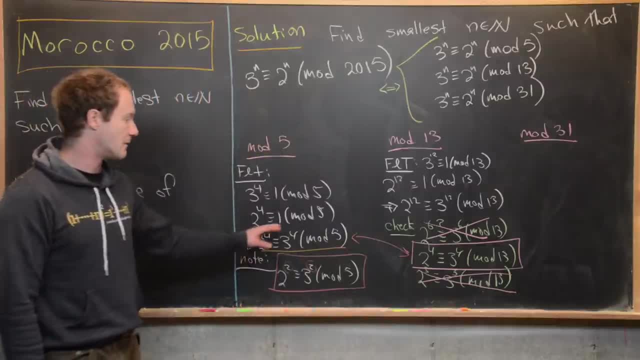 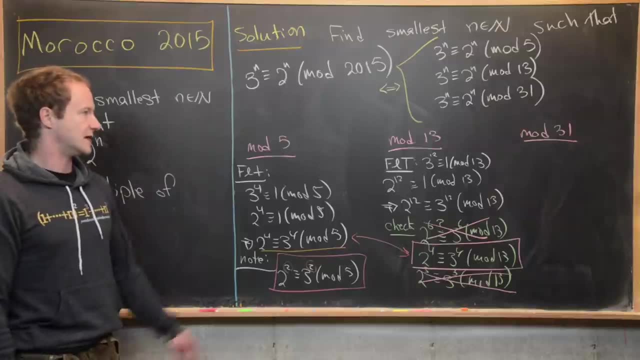 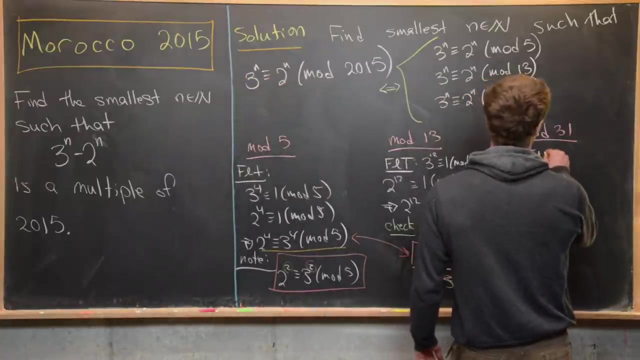 we can see that two to the four is congruent to three, 3 to the 4, mod 5 times 13 or mod 65. So we're actually part of the way there already. So now let's work mod 31. and so if we work mod 31, again using Fermat's little theorem, we know that 3 to 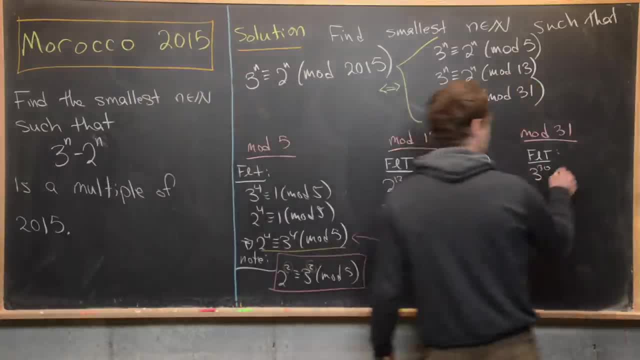 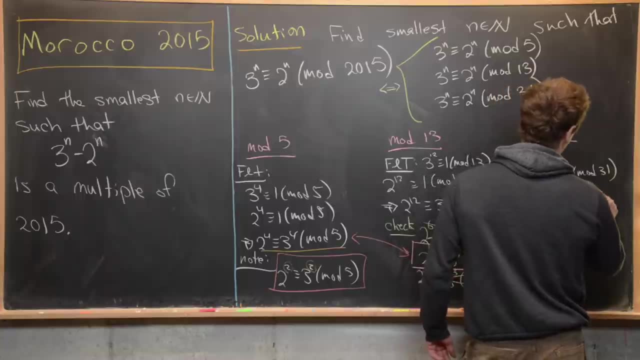 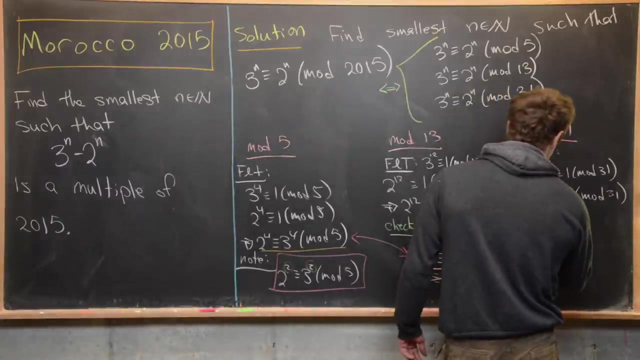 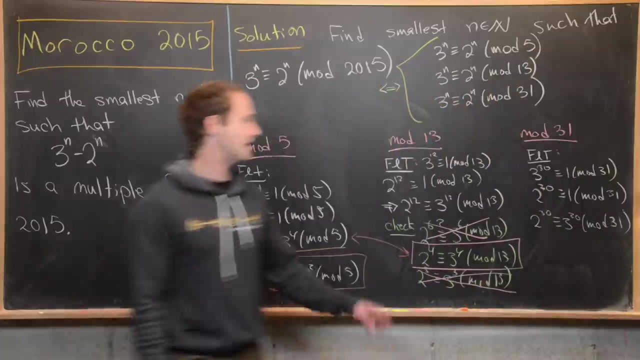 the 30, which is 31 minus 1, is going to be congruent to 1 mod 31, and then 2 to the 30 is also congruent to 1 mod 31.. Great, but that tells us that 2 to the 30 is congruent to 3 to the 30 mod 31, and then 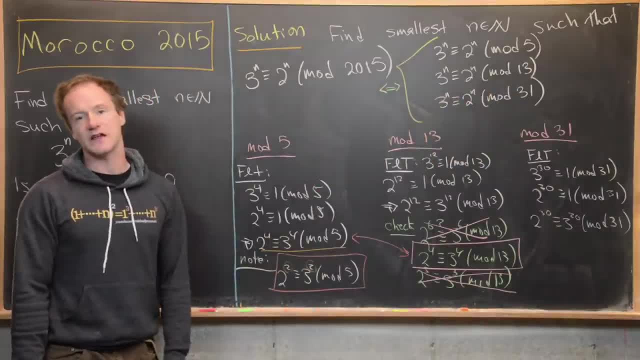 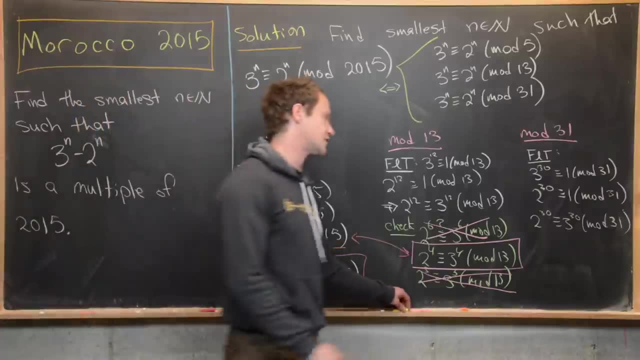 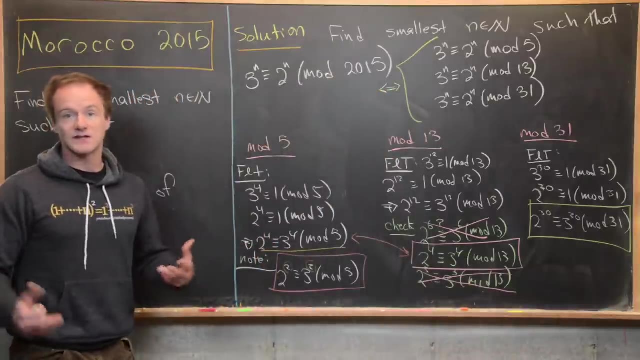 what you can do after that is check that none of the other cases work. So again, I'll let you guys maybe check that none of the other cases work, and so we land at this value right here. So this allows us to form our first good guess for the smallest value of n, and we'll check that. 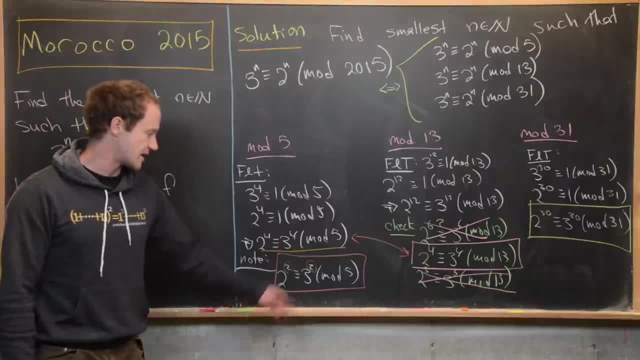 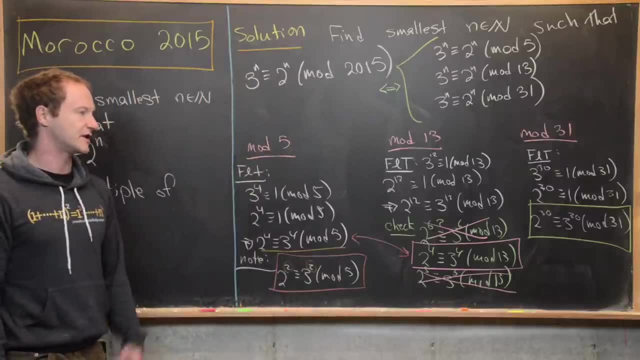 this guess works carefully. So notice, we've got: 2 squared is congruent to 3 squared, mod 5.. 2 to the 4th is congruent to 3 to the 4th, mod 13. and finally, 2 to the 30 is congruent to 3 to the 30. 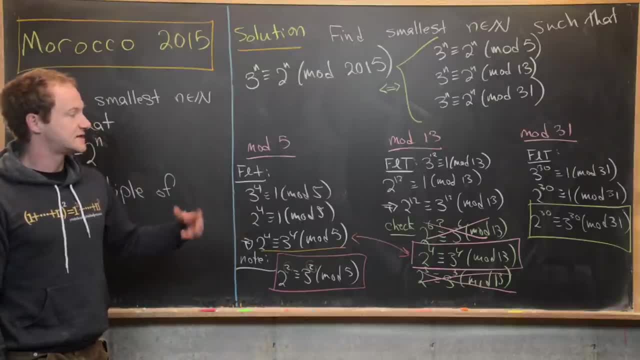 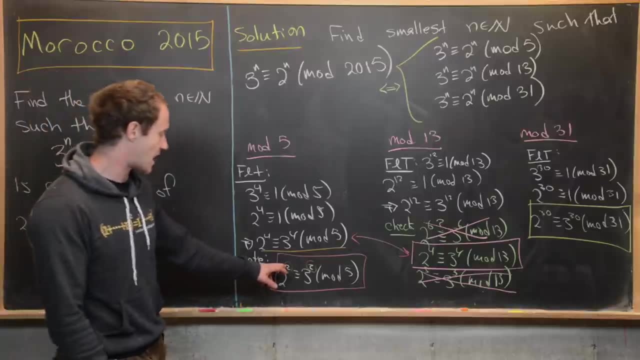 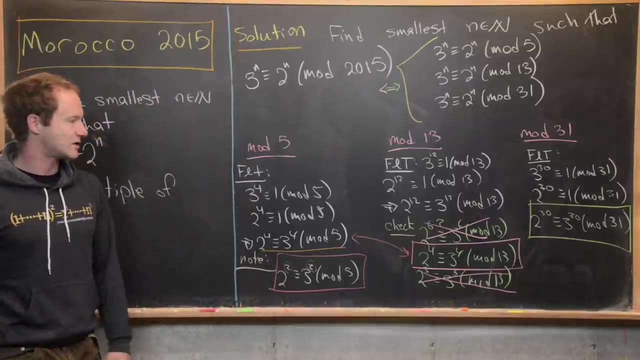 mod 31.. So, since raising an exponent to an exponent works multiplicatively, that gives us some of these three exponents, In other words 2,, 4, and 30.. The least common multiple of 2,, 4, and 30 is: 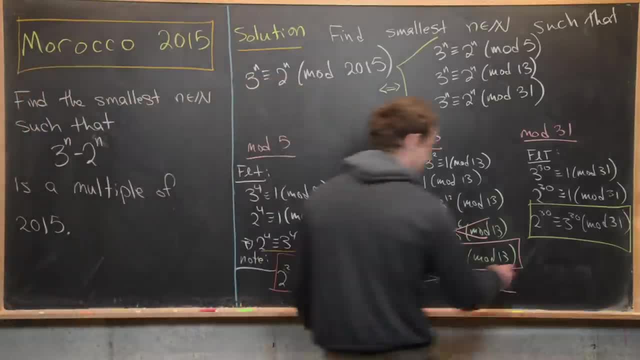 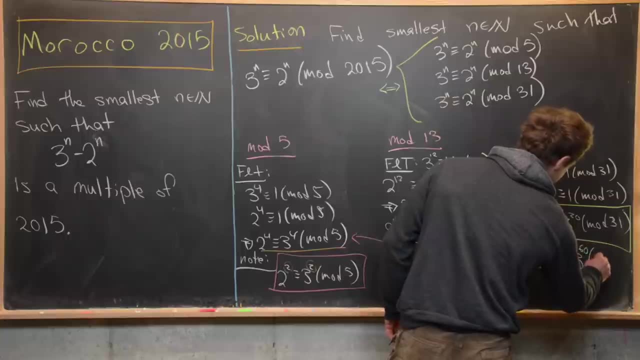 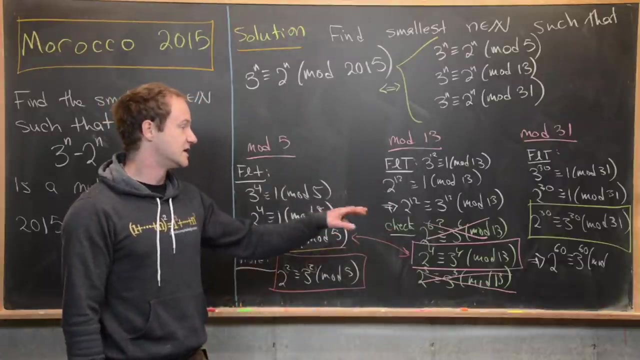 equal to 60. So from these three boxes here we immediately have that 2 to the 60 is congruent to 3 to the 60. mod well, mod 5,, mod 13, and mod 31.. That means 2 to the 60 minus 3 to the 60 is divisible. 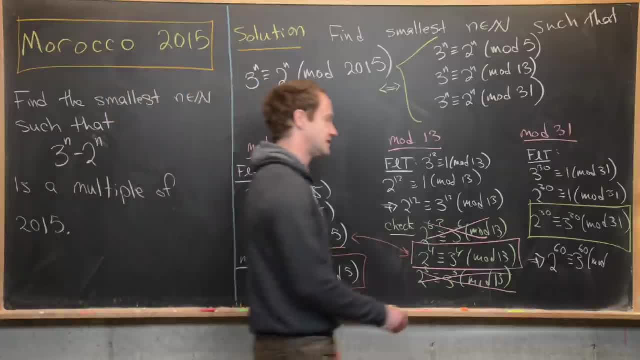 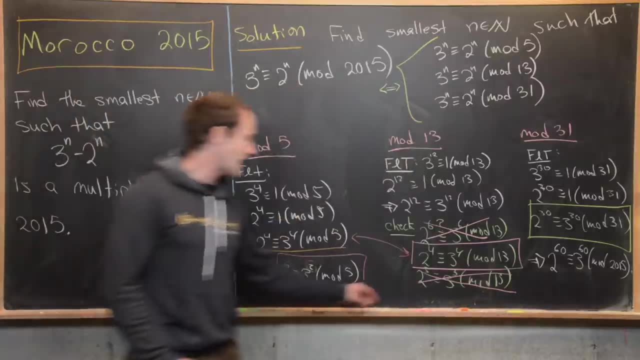 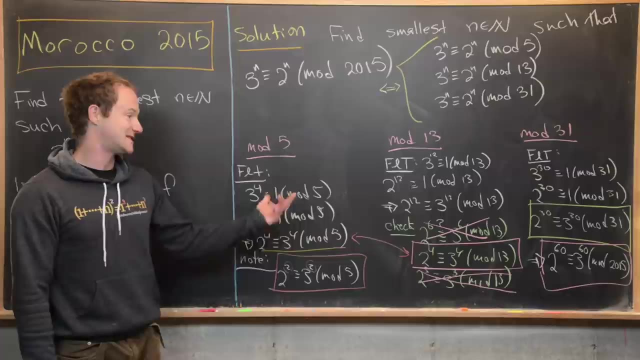 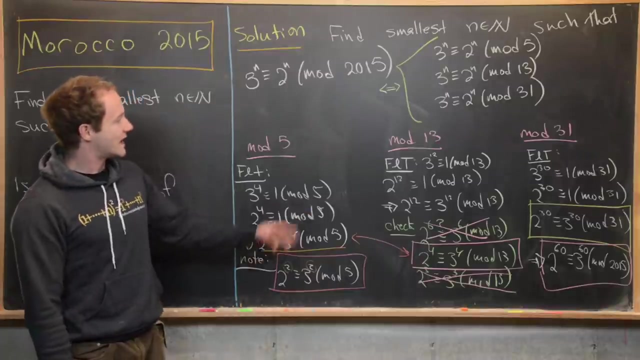 by 20 and 15, but that's the same thing as these being congruent modular 2015.. So we have proven this thing, which I'll box in pink over here, but what we don't know yet is that 60 is the smallest such exponent that allows us to get at this solution. So I'll go ahead and clean up the 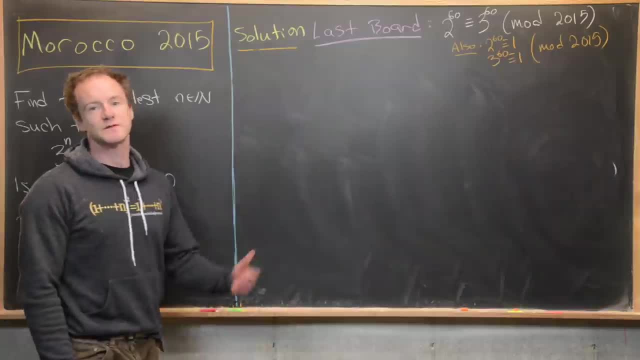 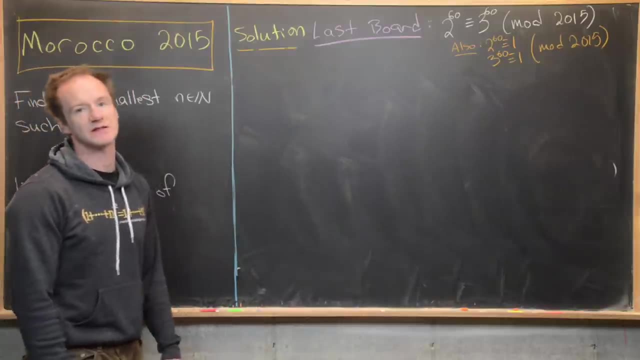 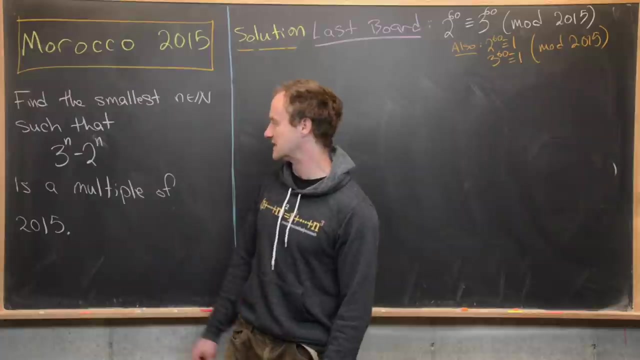 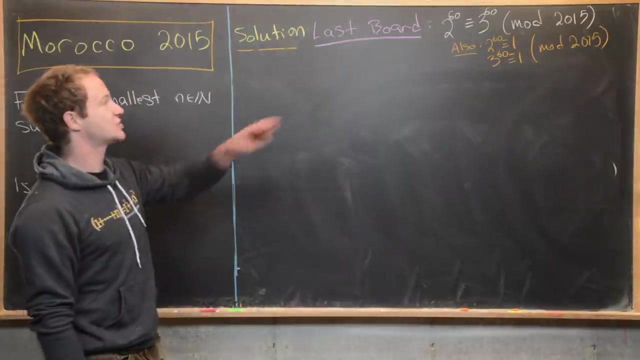 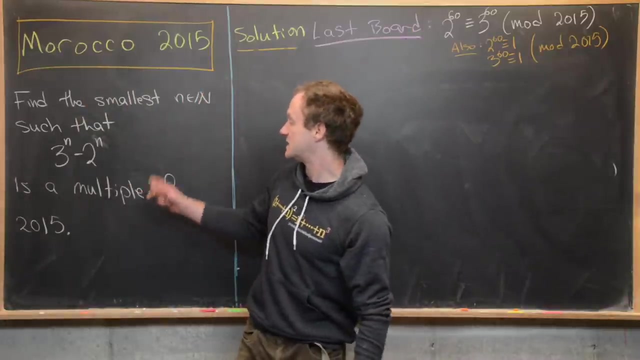 board, and then we will show that 60 is indeed the smallest. So, on the last board, we are going to see that 60 is the smallest such exponent, which will give us this congruence and thus give us this fact that we have this object as a multiple of 2015.. 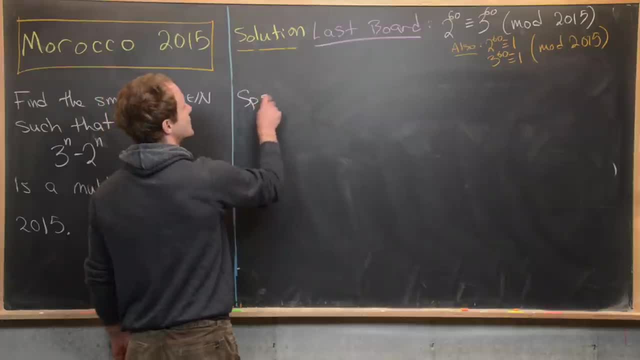 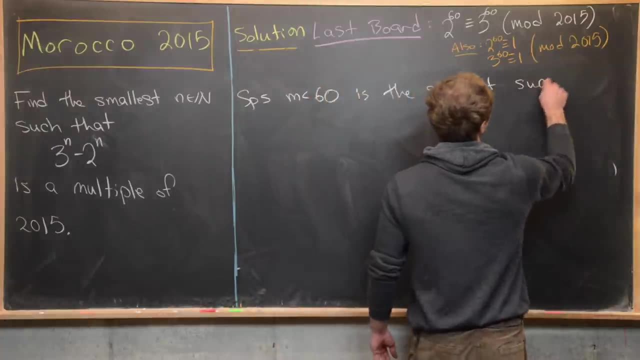 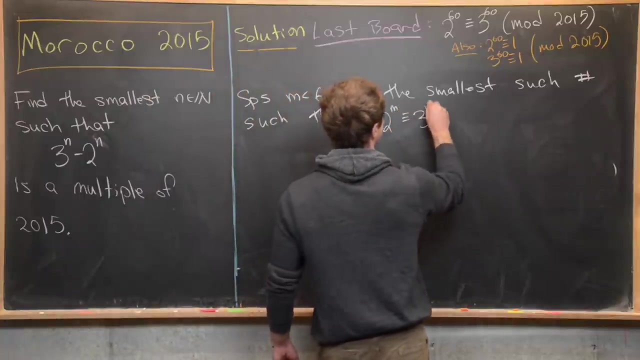 So let's see how to do that. So let's go ahead and suppose m is less than 60 is the smallest such number, such that 2 to the m is congruent to 3 to the m, mod 2015.. In other words, we want to. 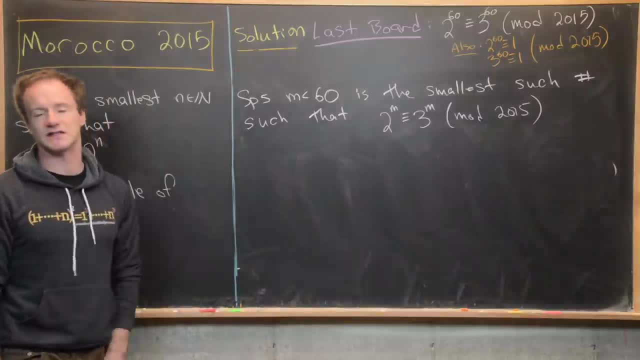 suppose we've got a number smaller than 60 that satisfies this congruence and furthermore, take the smallest such number that satisfies this congruence, Okay, cool. Next, we're going to do something which is a pretty common trick when it comes to these number theory type problems, and 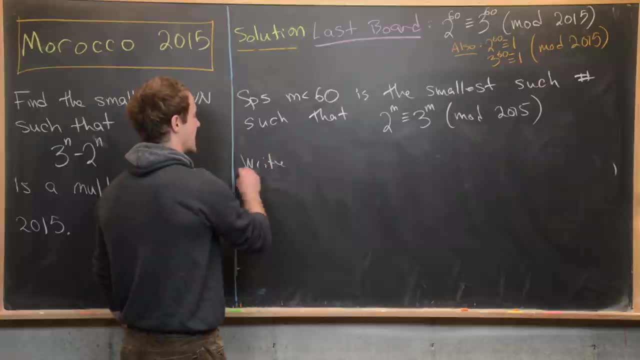 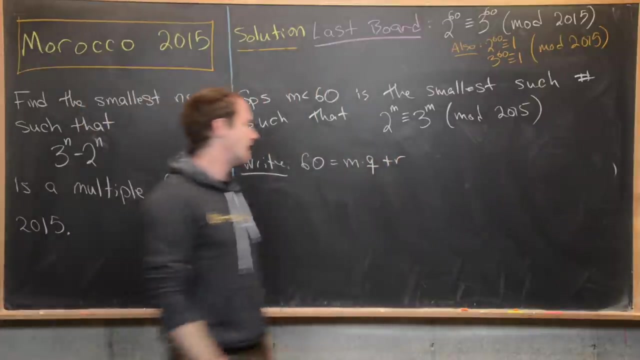 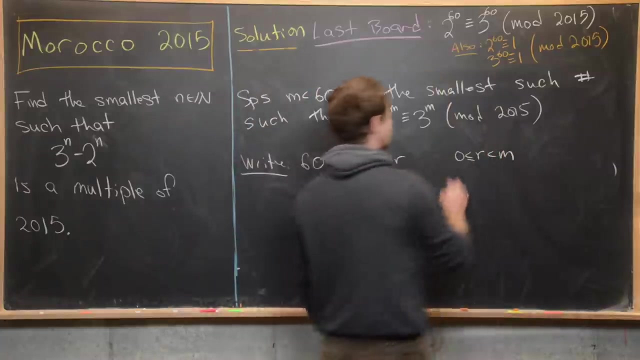 that is division with remainder. So let's go ahead and divide 60 by m and get the quotient and remainder. So this is sometimes called the division algorithm. So we can write 60 as m times q plus r, and here we know that r is between 0 and m. It's allowed to be equal to 0, but it is not allowed to. 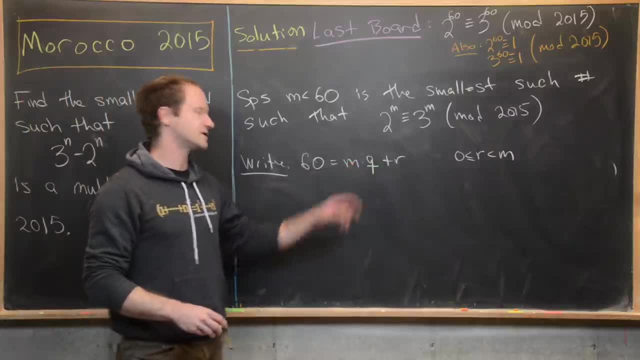 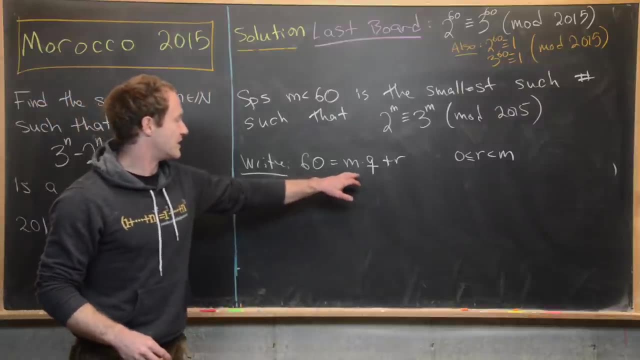 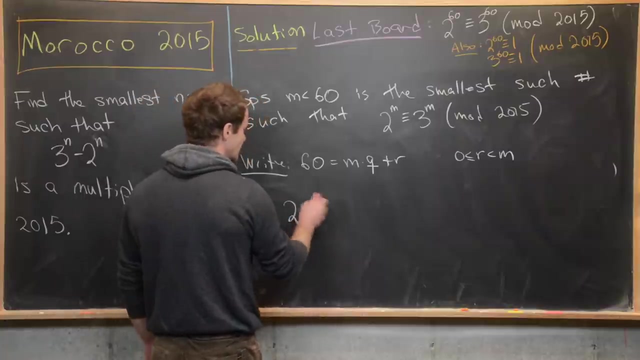 be equal to m. This is the remainder. like your remainder is always less than your divisor. Okay, so now what we want to do is insert this version of 60 into this congruence up here. So notice that's going to give us 2 to the 60, but I'm going to go ahead and divide 60 by m, So we're going to. 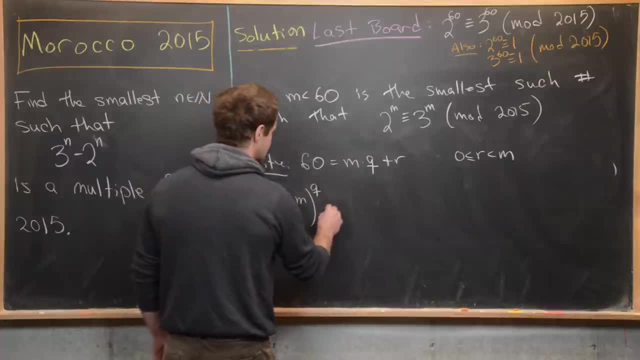 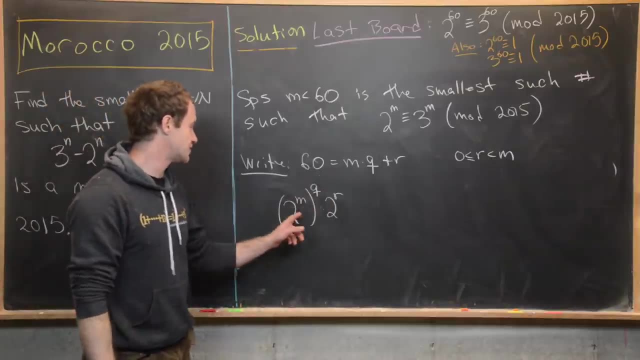 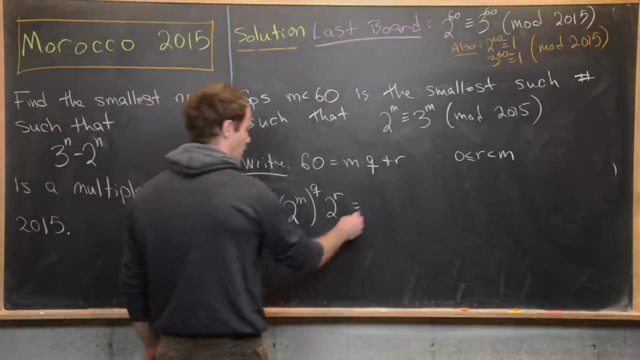 write that as m all to the q power times 2 to the r Again. I just use exponent rules there to change the multiplication to repeated exponentiation and so on and so forth, And then we've got the same kind of thing happening over on the right hand side. So here we. 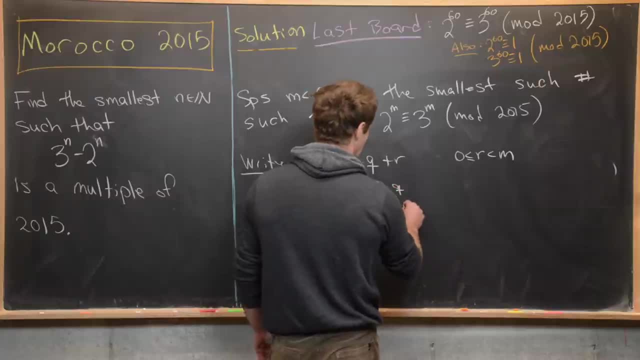 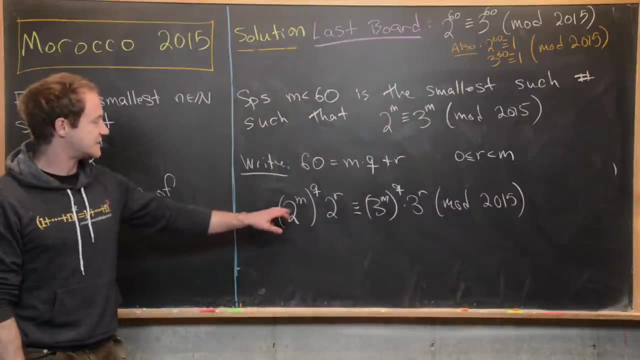 have 3 to the m to the q times 3 to the r and these are congruent modulo 2015.. But now notice that 2 to the m times 2 to the r is equal to 0. So we're going to write that as m all to the q power. 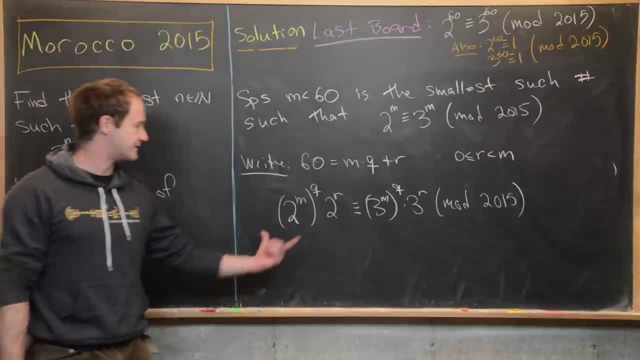 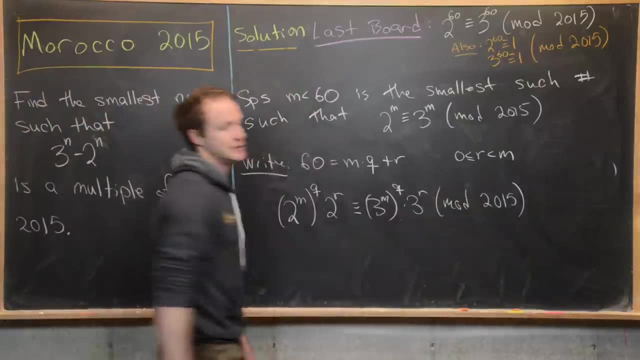 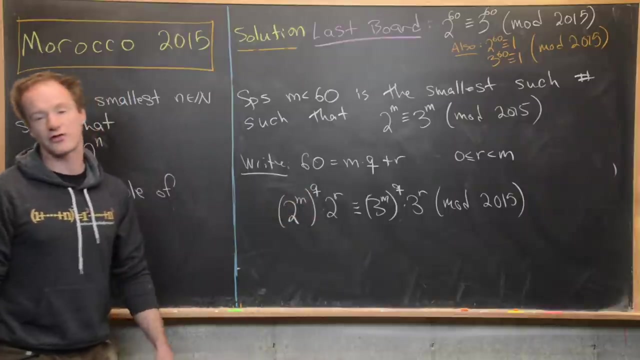 times 2 to the m and 3 to the m are congruent modulo 2015.. So these two are the same number And, furthermore, neither of them are divisors of 2015.. So that means you can cancel them from both sides. So that's actually pretty important that 2 and 3 are invertible mod 2015.. So that 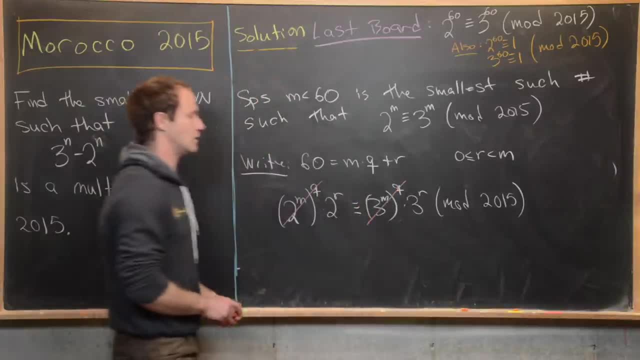 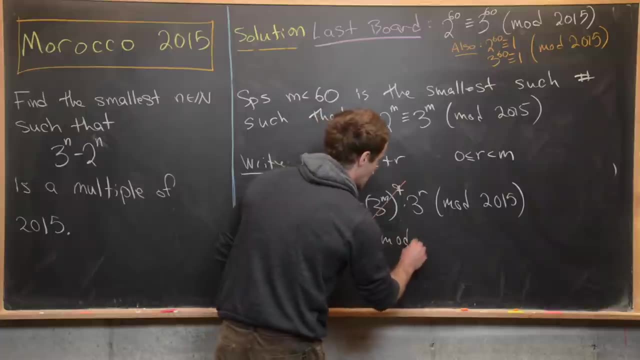 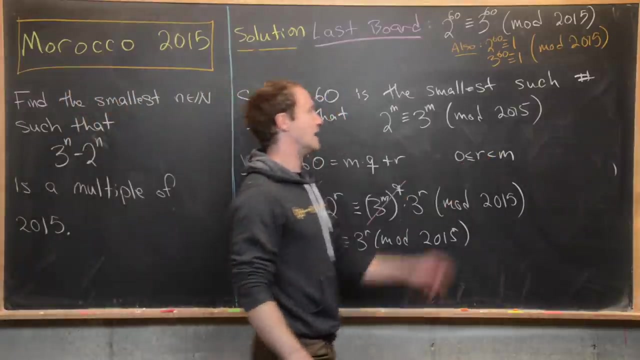 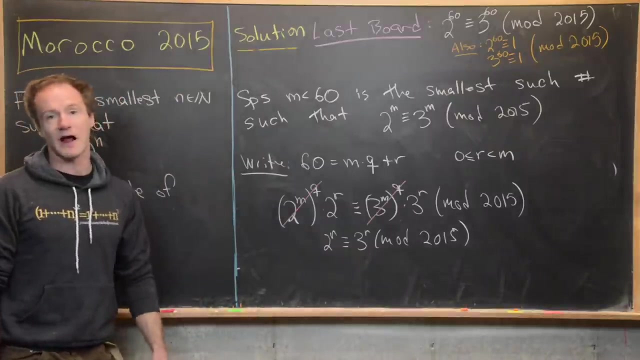 means we can cancel this whole thing, and this whole thing, leaving us with 2 to the r, is congruent to 3 to the r, mod 2015.. But let's see what we've got. We've got a number smaller than m that satisfies this exponential equation, But what that tells us is that number has to be equal to. 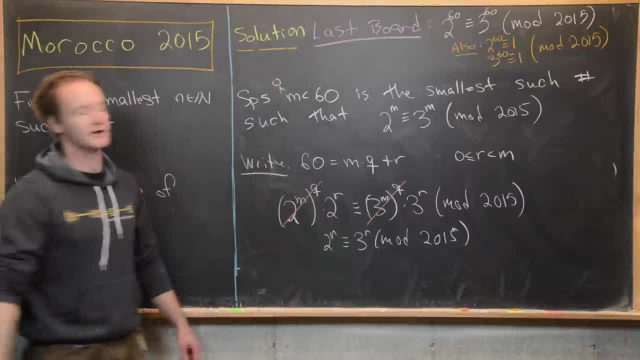 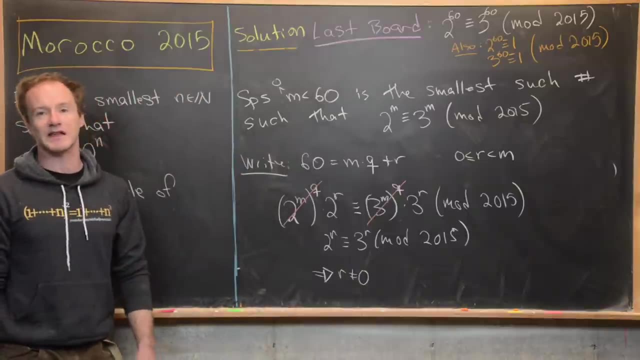 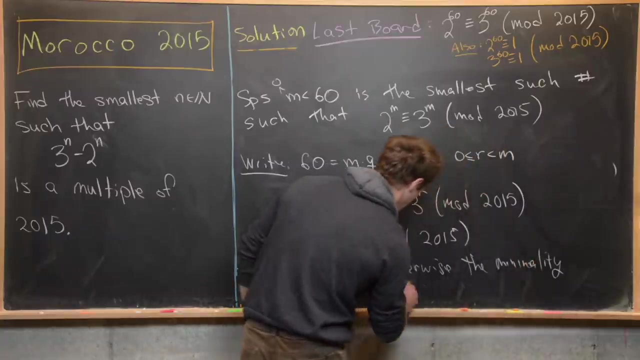 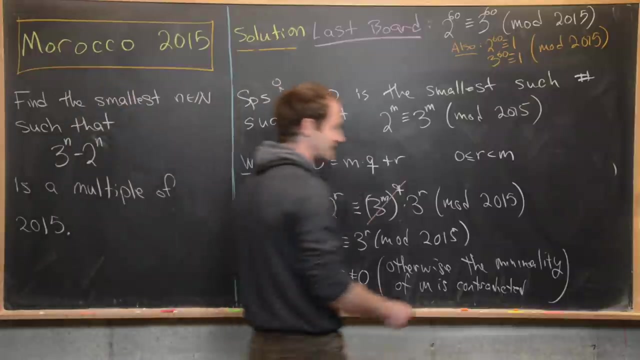 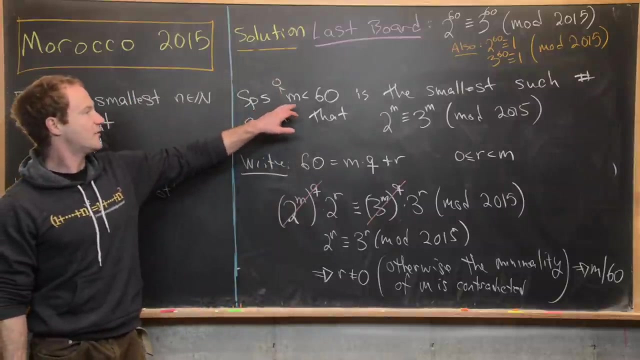 0. I guess I should say here that this one is strictly bigger than 0. Because otherwise we would contradict the minimality of m. Maybe write that down, Otherwise the minimality of m is contradicted, Okay. well, that's actually really good news, because what that tells us is that m divides 60. So in other words, if we have 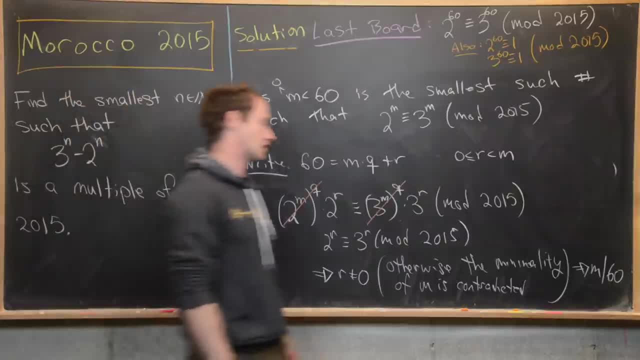 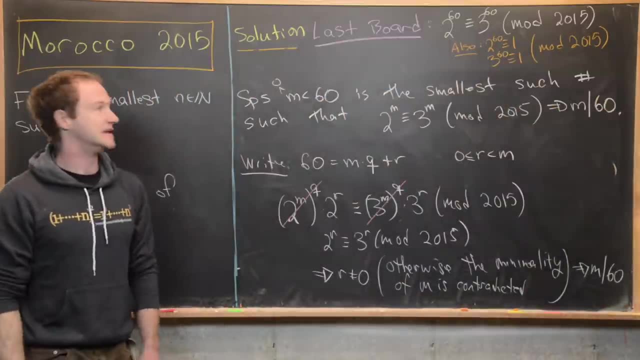 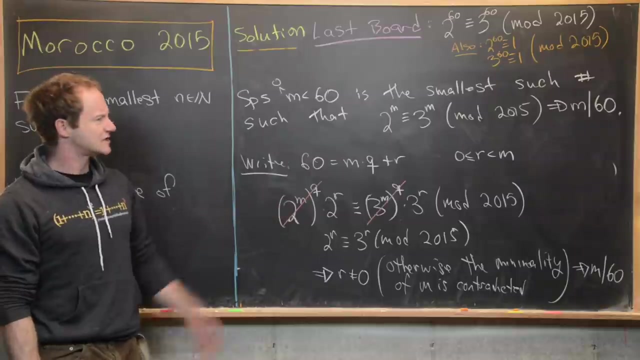 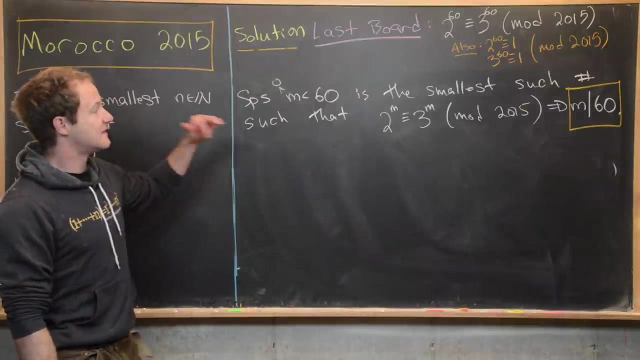 a number that also satisfies this exponential congruence. we know that that number must divide 60. Given that 60 already divides that exponential congruence, Okay, so I'm going to maybe like clean up the board from here down and now it's just the case of checking all of the divisors of 60.. On the last board, we noticed 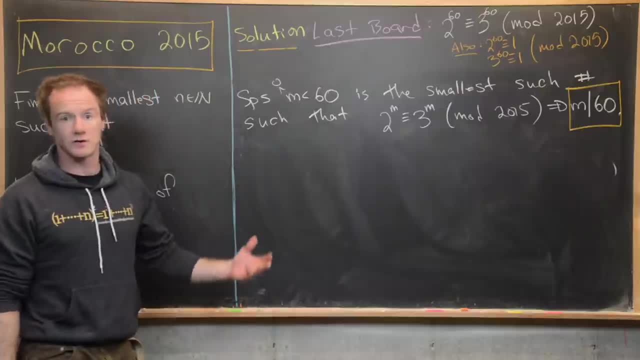 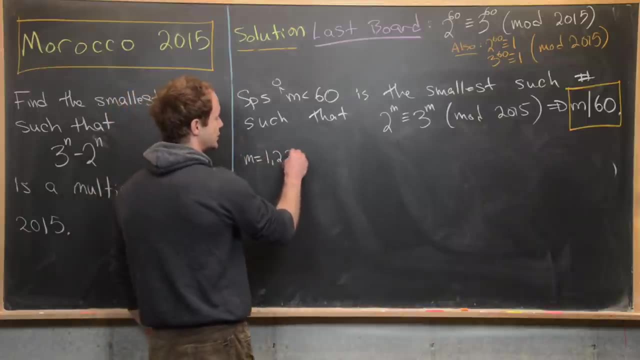 that if m satisfied this congruence, then m had to be a divisor of 60. So what that tells us is that m can be equal to 1,, 2,, 3, 4.. Let's see: 5 is a divisor of 60.. 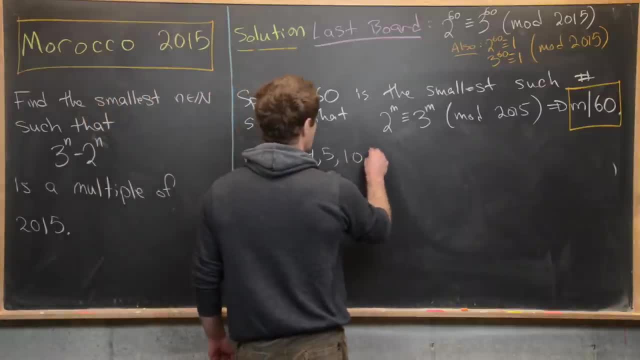 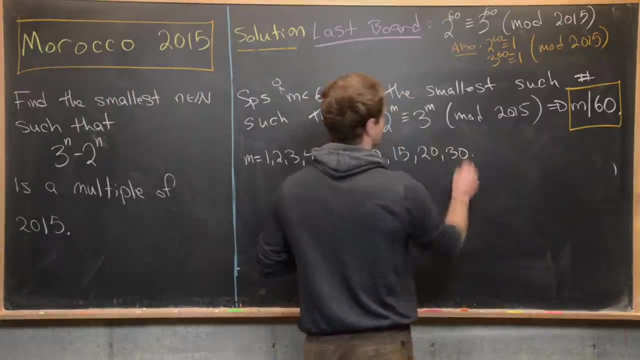 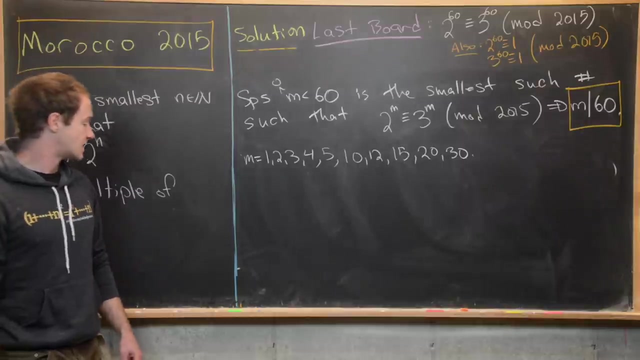 Let's see what else. 12 is a divisor, Well, 10.. And then 12 is a divisor of 60. And then 15,, 20, and 30. So those are all divisors of 60. So we want to make sure that none of those work, So I'll do a. 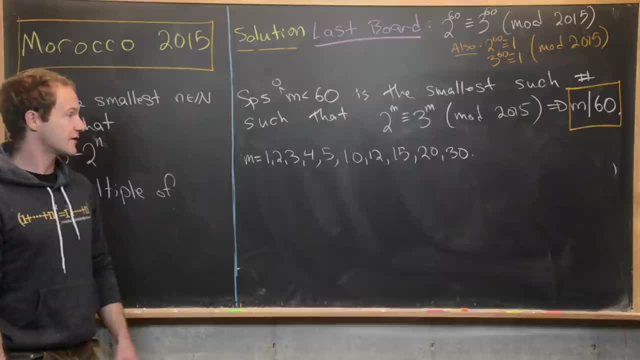 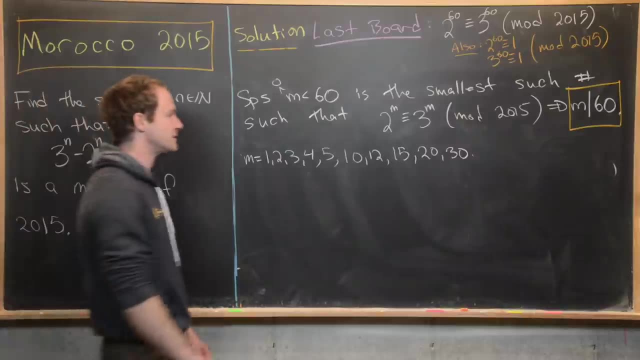 couple of them and then I'll leave you guys to do the other ones. I will say that there is a trick here, but I don't really want to get into it because that we've used enough technical tricks here, So let's maybe go ahead and do that. 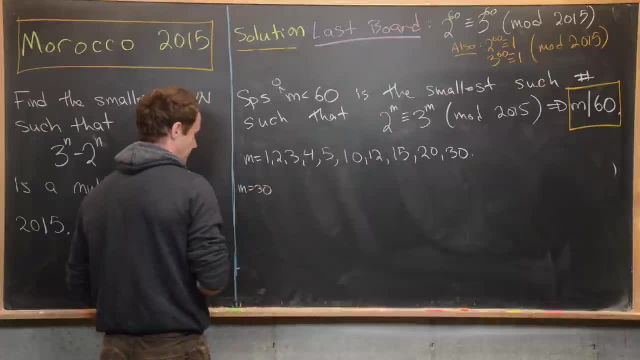 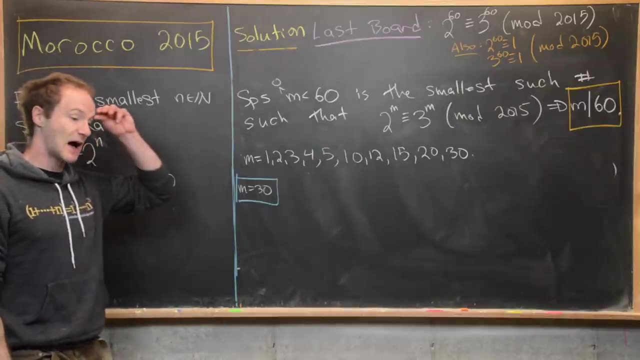 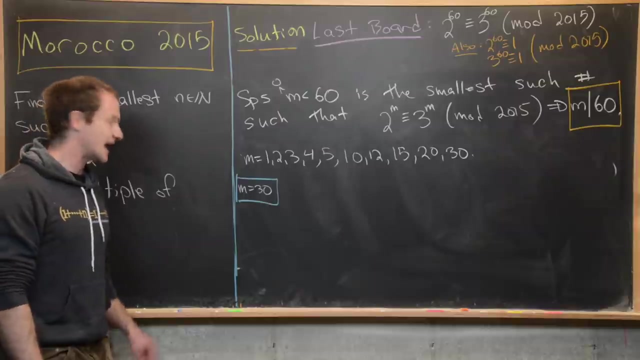 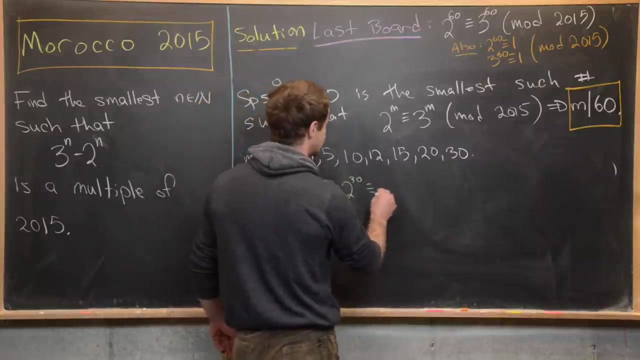 Go ahead and check m equals 30 first, And so I am not going to work modulo 2015.. I'm going to be inspired by what I saw when I was working modulo- the prime factors- to guess where this goes wrong. So let's maybe recall that 2 to the 30 was congruent to 3 to the 30 modulo 31.. 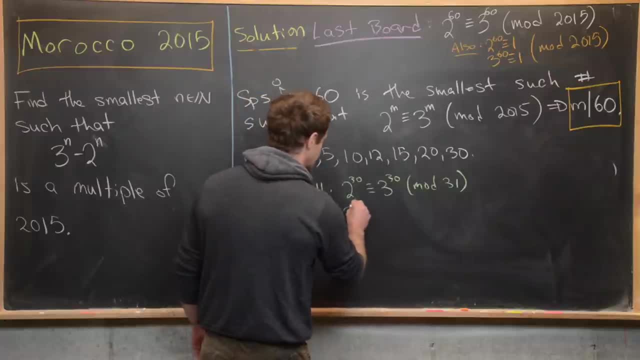 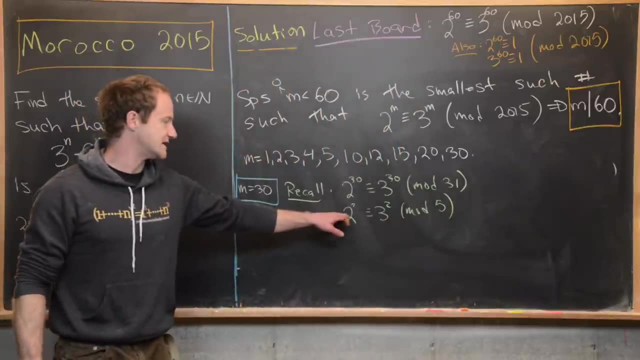 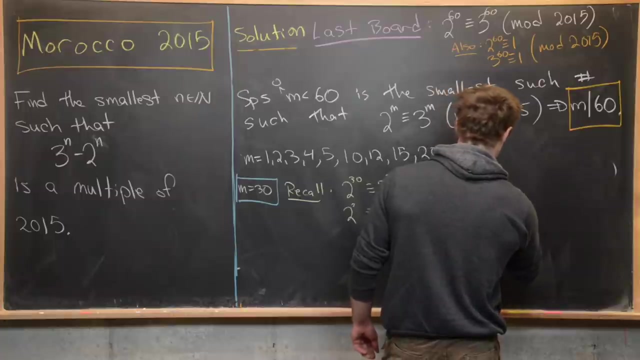 Great, And 2 to the 2 was congruent to 3 to the 2 mod 5.. But now what we can do is raise each of these to the 15th power, And that tells us that 2 to the 30 is congruent to 3 to the 30 modulo 5.. 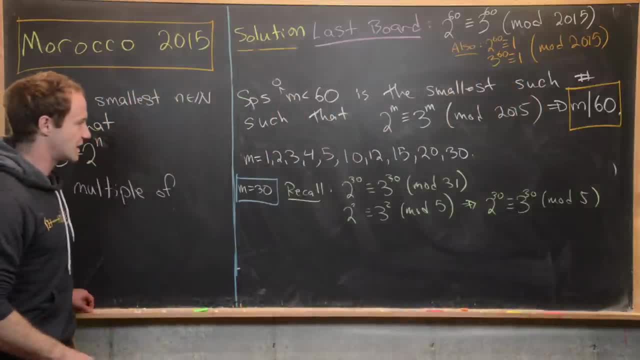 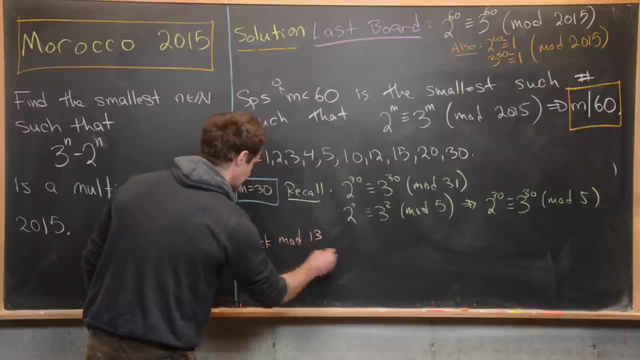 So all we really need to do is check what's going on. modulo the remaining prime, In other words 13.. So check mod 13.. In other words, we want to calculate 2 to the 30 and 3 to the 30 mod 13.. 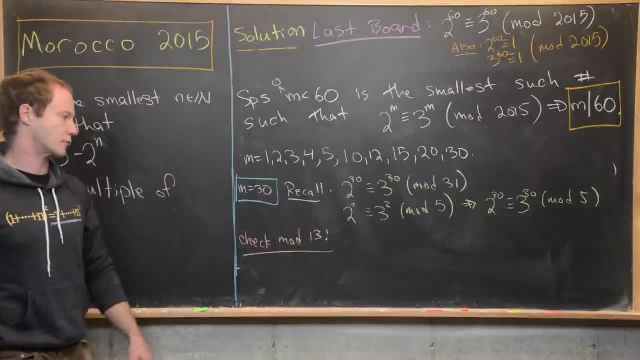 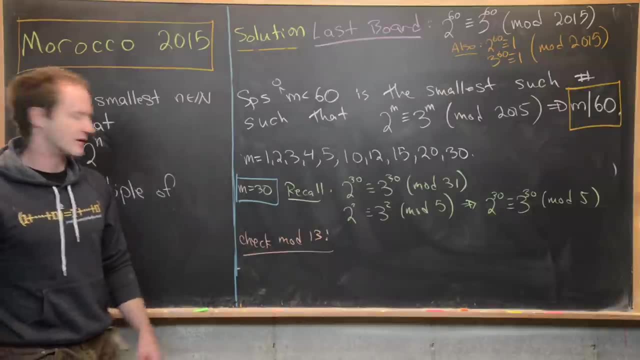 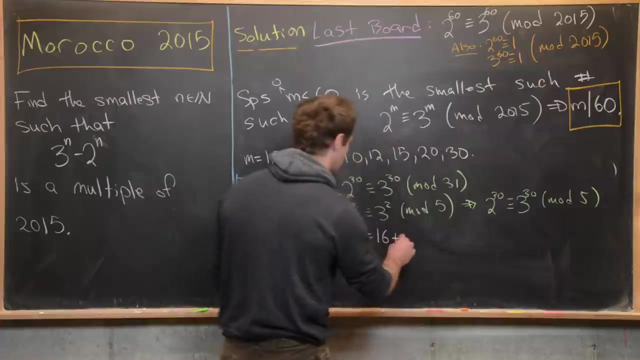 And there's actually a trick for doing this. It's called the method of repeated squaring, And so what it involves is writing 30, basically in its binary representation, or as a sum of powers of 2.. So, notice, we can write 30 as 16 plus 8.. So let's see. 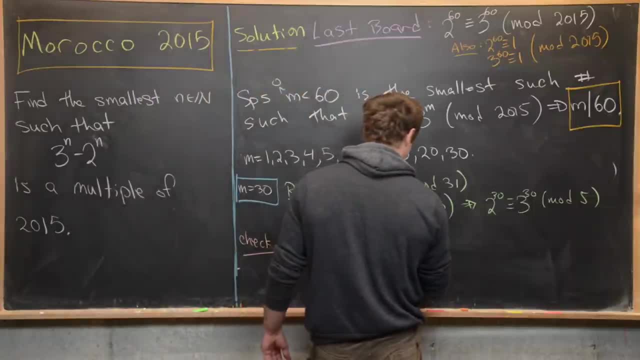 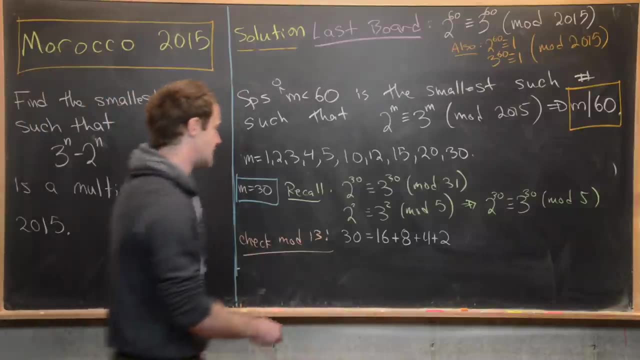 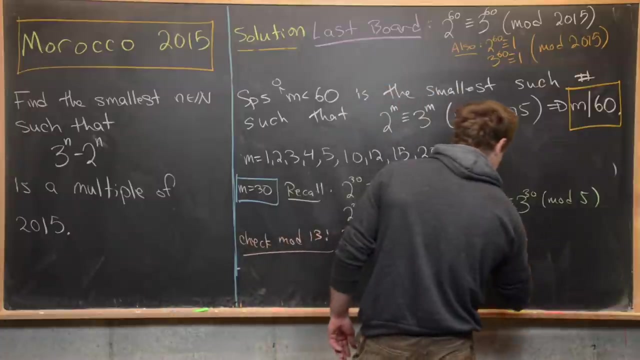 Let's see So if this changing here- what is at 15 plus 8, is going to be 24.. And then we're going to add 4 and then a 2.. Great, So what that tells me is really what I really need to calculate: 2 to the 30,, which is going to be the same as 2 to the 16 people, as 2 to the 8, times 2 to the 4, times 2 to the 2, and I want to compare that to: 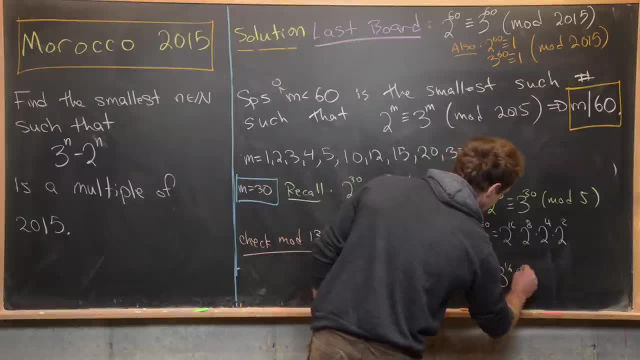 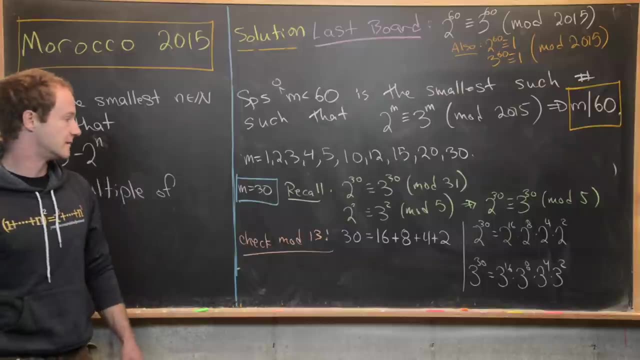 3 to the 30, which is 3 to the 16 people- Great 16. 3 to the 8, 3 to the 4 and 3 to the 2. okay, good, and again we're working mod 12 in all of these. 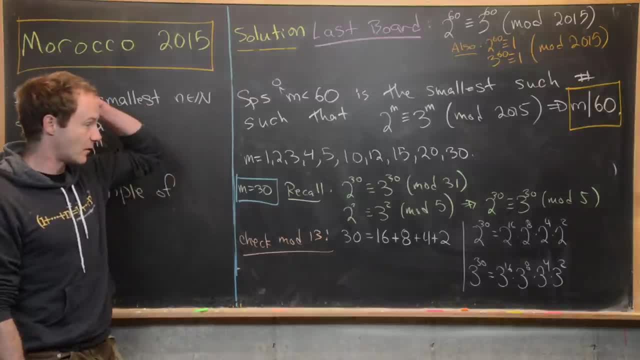 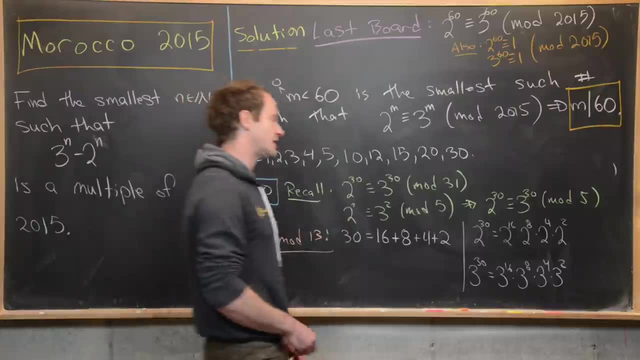 so next i want to recall from our calculations before that 2 to the 4 and 3 to the 4 were both congruent to 1 mod 13. so what that means is that this is congruent to 1 mod 13. this is also. 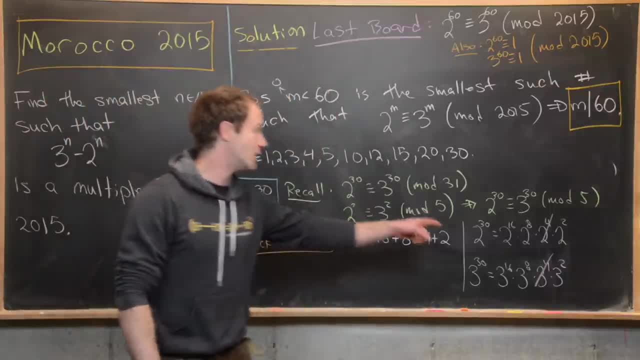 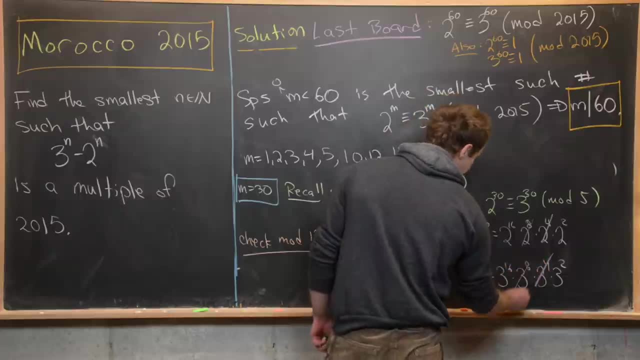 congruent to 1 mod 13 and then notice that this is going to be 1 squared because it's 2 to the fourth squared. so this is also congruent to 1 mod 13. this is also congruent to 1 mod 13. 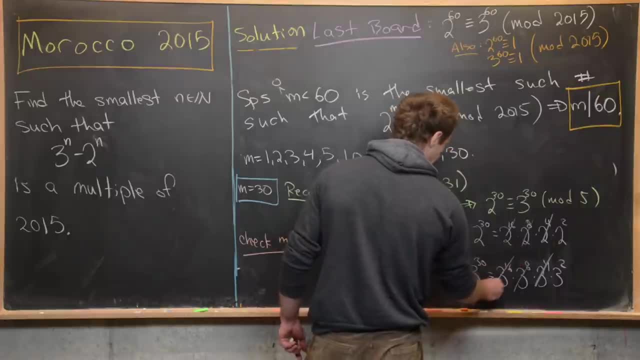 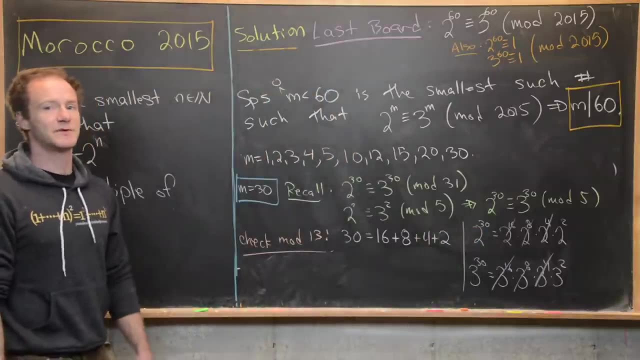 and finally, this is congruent to 1 mod 13. and this is congruent to 1 mod 13 again because this is going to be like 1 to the fourth power, but now we can simplify our calculation quite a bit. so let's notice that 2 to the 30 is going to be congruent to 2 squared. 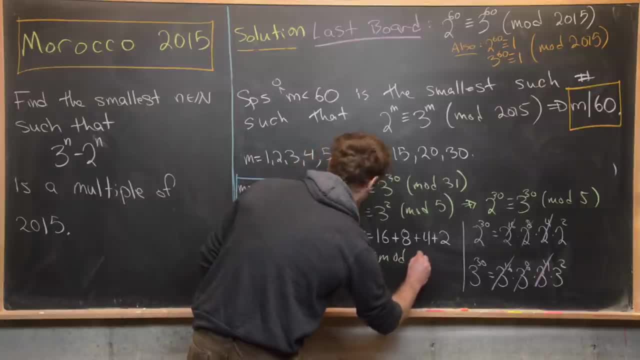 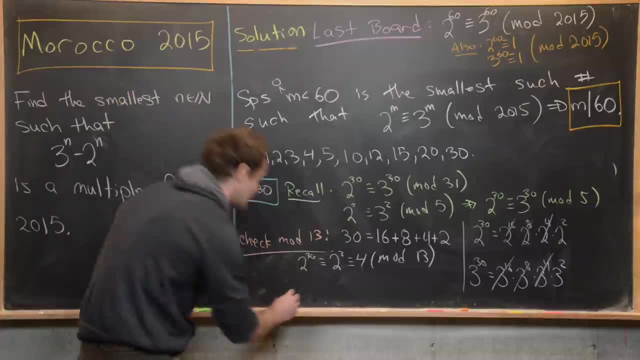 which is congruent to 4 mod 13. again, because all of these parts are congruent to 1 mod 13, but then 3 to the 30 is going to be congruent to 3 squared, which is going to be congruent to 9. 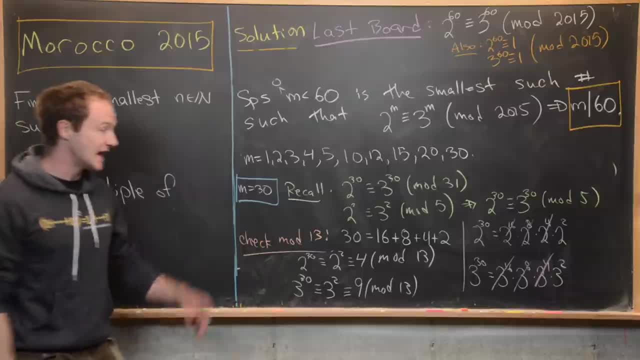 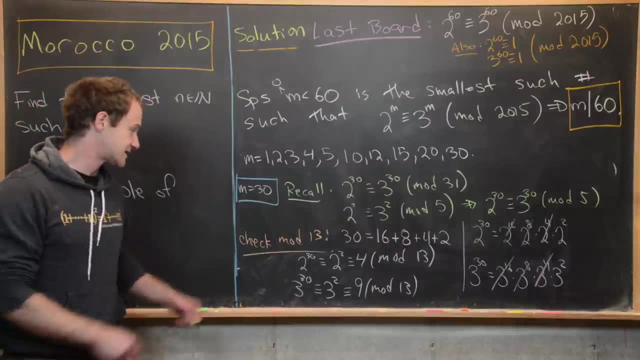 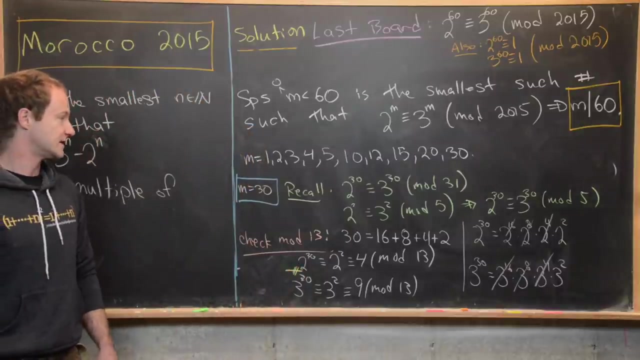 mod 13 again, because all of these parts are congruent to 1 mod 13.. So what that tells us is that 2 to the 30 is not congruent to 3 to the 30 mod 13. but now putting that together with, 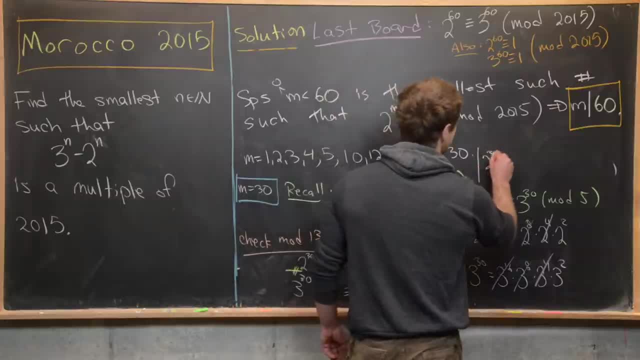 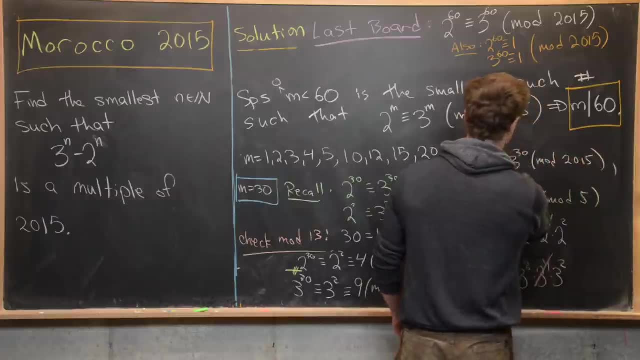 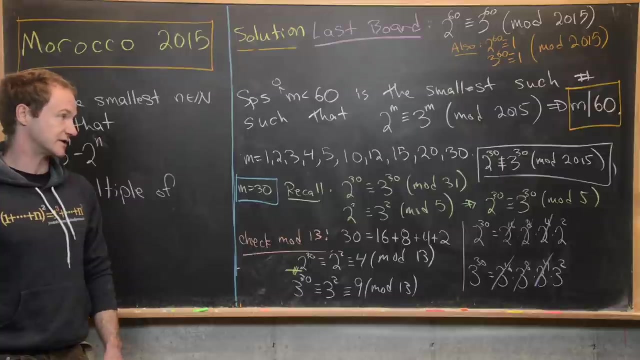 these. we see that that means that 2 to the 30 is not congruent to 3 to the 30 mod 2015, because if it were, then you would have congruence module all of its primes, including 13.. So what we've done? 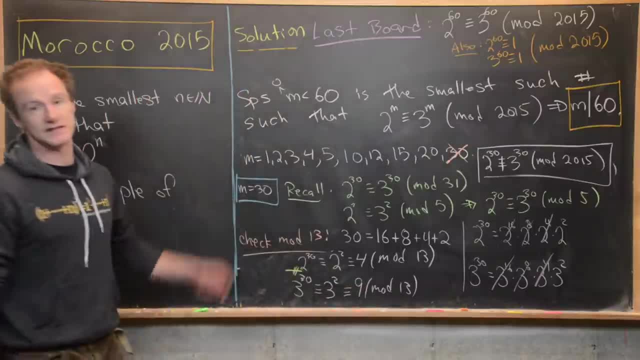 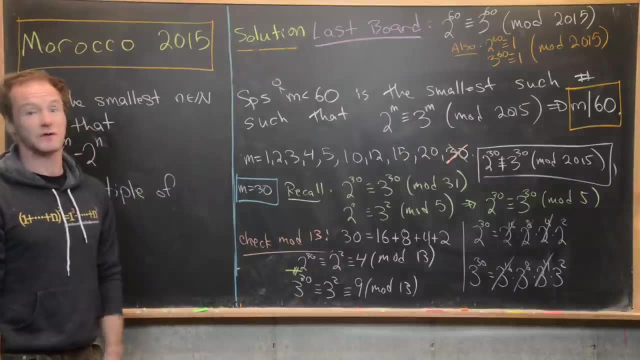 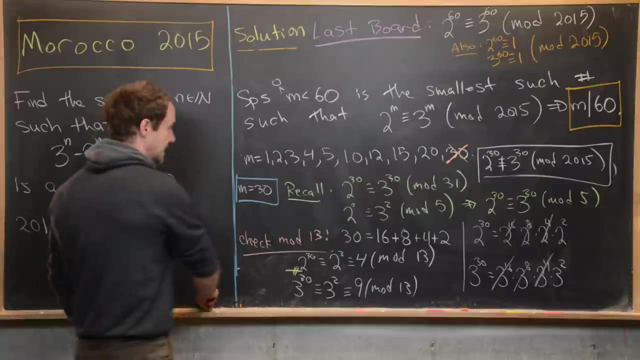 is eliminated 30 from the possibilities here, and then you're just going to want to do that with all of the rest of the possibilities and see that none of them works. So I'm not going to go through that. you can go through that using the same sort of calculation, but what you'll see? 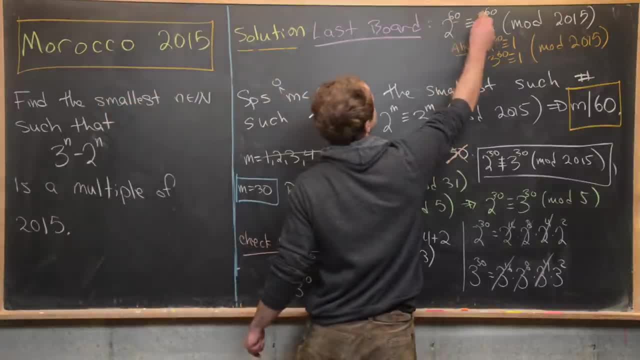 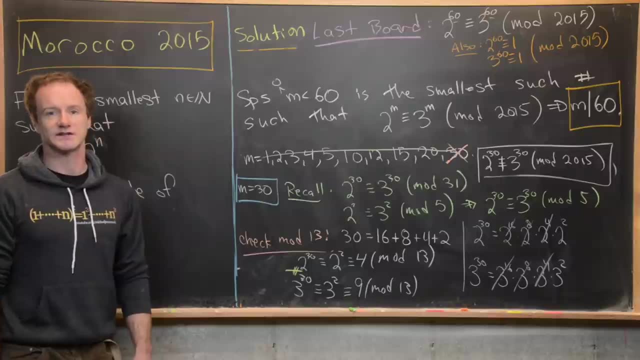 is that none of these are okay, which tells us that this 60 up here is, in fact, the smallest such exponent. that allows us to finish this off, and that's a good place to stop. Subtitles by the Amaraorg community.